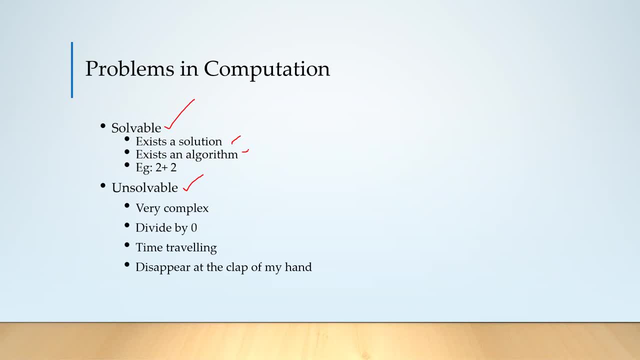 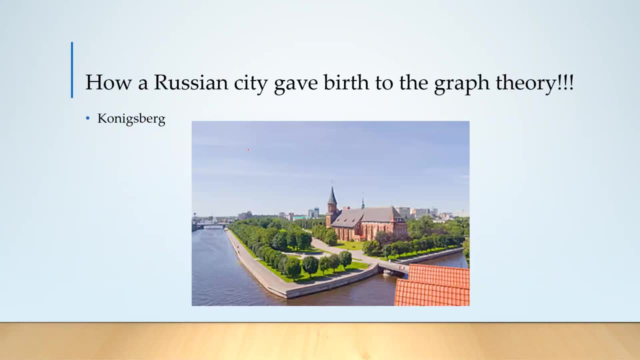 they can either be solvable or they cannot be unsolvable. now, before we go into detail about solvable and unsolvable problems, uh, there's a very pretty picture over there. uh, it is the city of konigsberg. the city of konigsberg it is. it was in prussia, uh. now, uh, it is in the current. 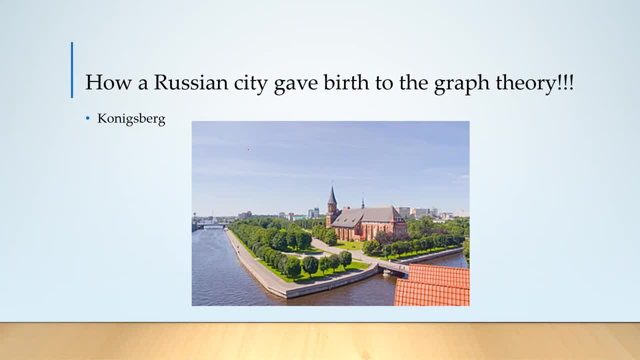 russia, a very beautiful city with a lot of water bodies, uh, and then small islands, markets and all a very pretty russian city. now, it is actually in this russian city of konigsberg that the graph theory took birth. now, in the city, uh, of konigsberg. 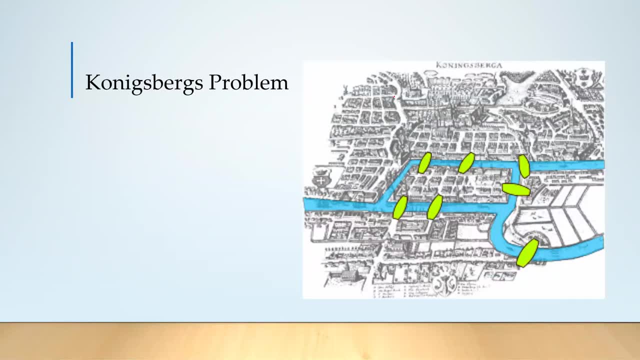 there were seven bridges, okay, what you see in blue, they are the water bodies, and then the things which you see in green, they are the bridges over there in konigsberg. okay, so you have these bridges connecting. okay, this part of the land and this part again. you have. you know, actually there were. 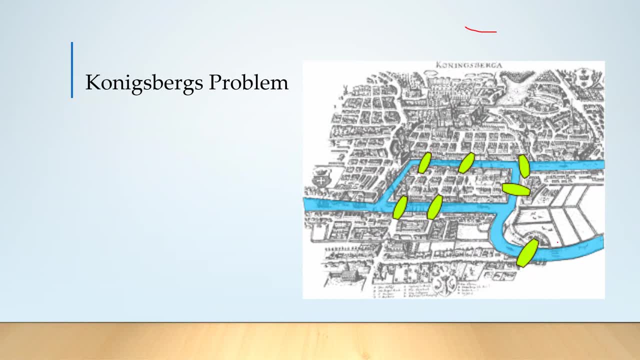 seven bridges: one, two, three, four, five, six, seven. uh, this is a picture of the 17th century. now, all these bridges are not dead. there was the world war and all that, and then you have the water bodies. many of the bridges have gone. some bridges were renovated. i think only, uh, two, three bridges of. 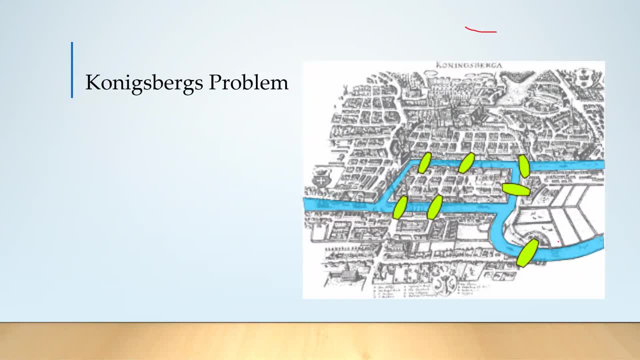 the original seven bridges are there, but anyway, this is where the original graph theory took birth. there was a city of konigsberg, and then you had many bridges connecting the various lands, between the water bodies. and in uh, those times, those uh 17th century times, there was a game. 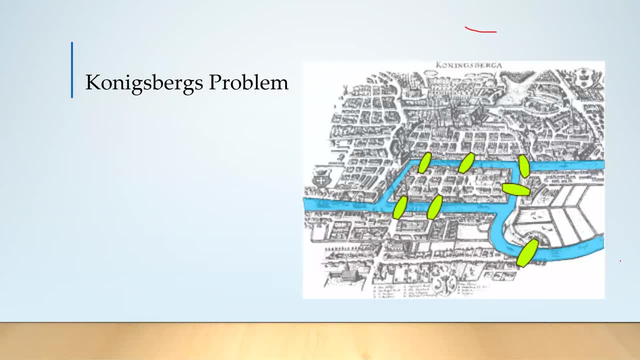 like you know, you start anywhere. you start in any piece of land. okay, let's say you start over here. okay, you start over here, travel through all the bridges, travel through all the bridges exactly once, exactly once, and then come back to the point where you started. oh my god. 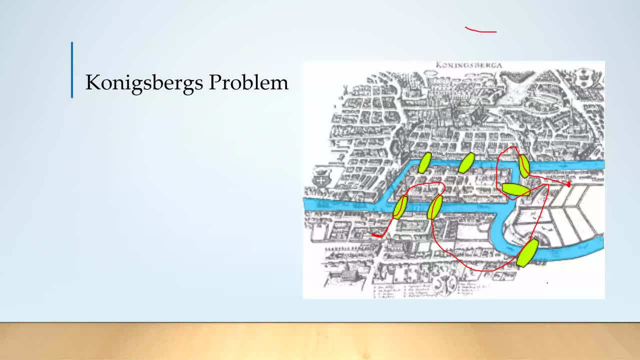 i wasn't. you know, i started over here, i started over here and then i ended up over here. i cannot, no, i couldn't, i couldn't. let me start a different way. i start over here. i come here, i go like this, i go like this, i go like this, this. oh, i again need to cross a bridge. you know, this bridge wasn't covered. 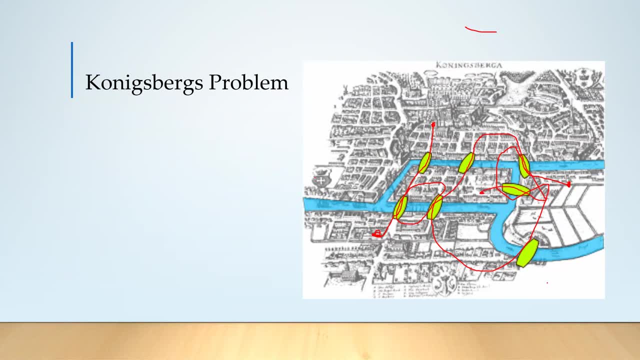 okay. so the question was: start in a particular point, travel through all the bridges exactly, exactly once and then come back to where you started. those days there were lots of bets with money, without money, and all that. it was a very popular game, like you know. people used to start. 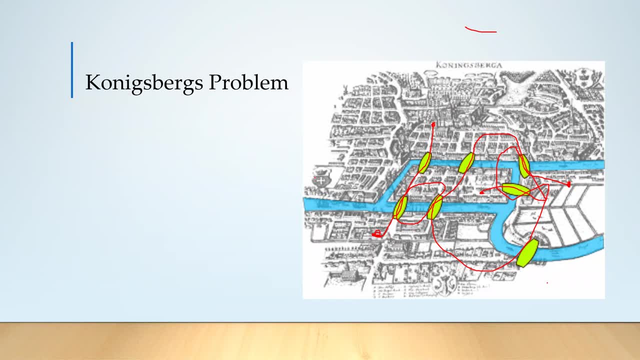 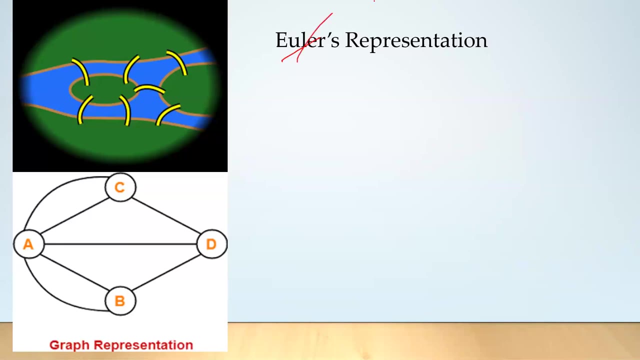 funding from one way to the other. and then you know, uh, people couldn't try completing the problem, starting at a point, coming back at the same point. but you know, you have to cross all these bridges. so that is when this man called Euler, leonard euler, leonard euler, he was a very great mathematician. he was a very great mathematician. 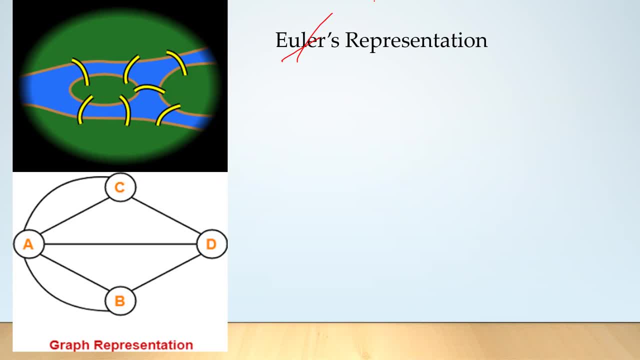 he's in fact called the king of mathematics, king mathematician, one among the greatest mathematician of history. uh, he not only was a mathematician, he was- uh, you know, he was almost well worst in all uh branches, like you know. think about geometry, calculus, algebra, trigonometry, number theory. 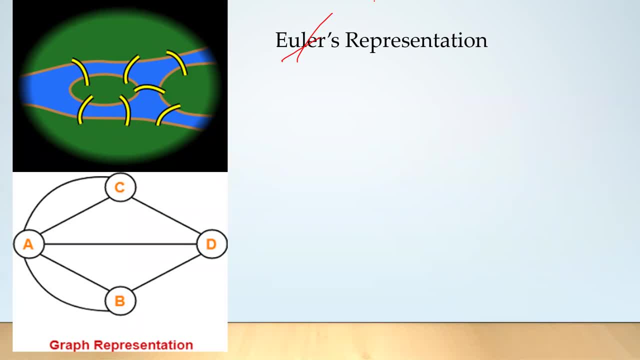 it physics, be it astronomy, whatever you know, euler was uh, euler was a genius anyway. so, uh, this man called euler, he thought, you know, uh, i need to find a solution for this, i need to find a solution for this and the bridges. he tried to uh bring about a structure, like you know, for the bridges, and then 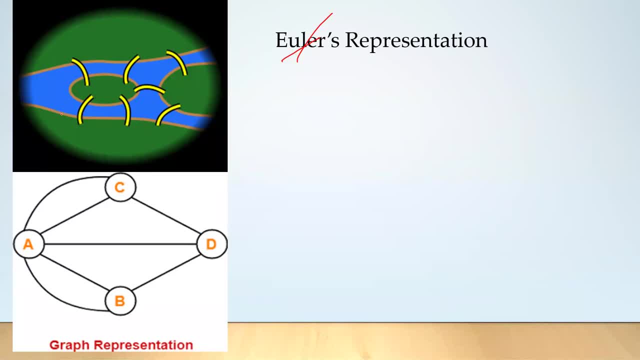 you know, he came up with a simplified structure, the one you see over here, in green, black and blue. and then, you know, the blue are the river, are the river bodies, and then the yellow are the bridges. so, you know, he thought, you know, i'll just name these, i'll name this a, i'll name this land body. 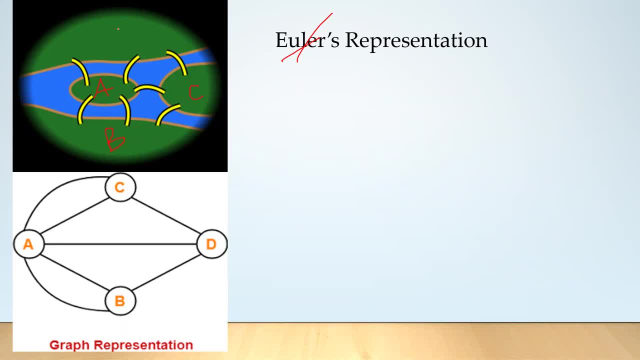 the land bodies. he just simply named it a, b, c, d, and then he came up with a simplified structure. he came up with a simplified structure, this a, this a. he gave it, you know, in a circle kind of a thing, a, and then he called this to be node or vertex. he called this to be vertex. 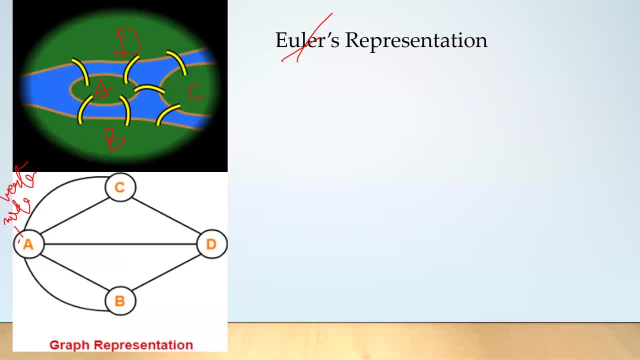 okay, and then a had five bridges going up, five bridges going out: one bridge, the second bridge, the third bridge, the fourth bridge and the fifth bridge, and then this particular konigsberg problem- call it the konigsberg problem- he was able to convert it into this kind of representation. where did he did have something? 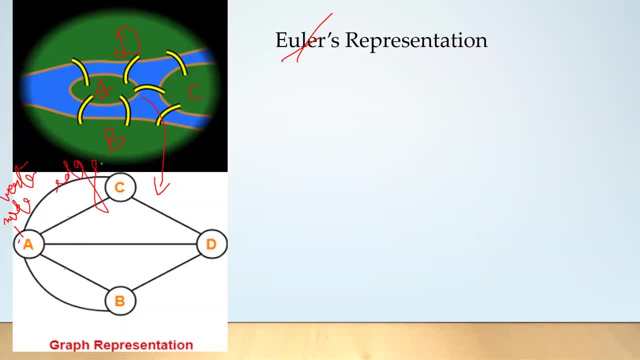 called vertexes, vertices, and then the edges. edges are nothing but the bridges, the bridges which connect a to c and so on. so this is how, actually, the graph theory came out. euler, he propounded the graph theory. he is actually the creator of the graph theory, and this is the first graph in history. 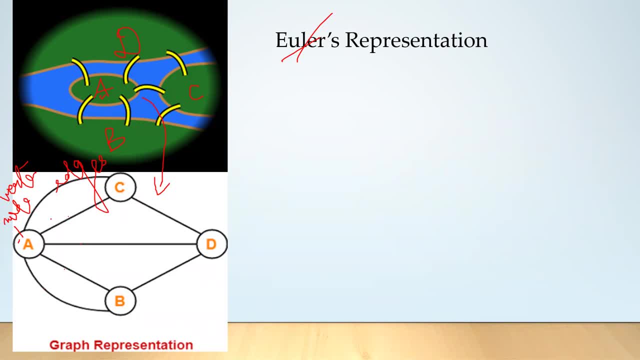 in mathematical history. this is the first graph from the konigsberg bridges. he was able to bring out this particular graph and now he bought out a representation. and now his question was: to solve the problem. now he, uh, tried solving the problem. the problem is nothing, but this start from a start, from a vertex, a go through each and every edge, go through. 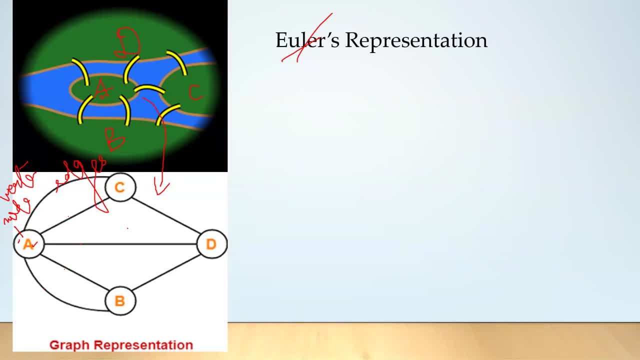 each and every edge. pass through the vertex only once. and come back to my starting point. okay, so there were three conditions. start from any vertex, come back to the vertex, pass each edge. sorry, pass each edge exactly once. and that is what came up to something called the euler cycle. 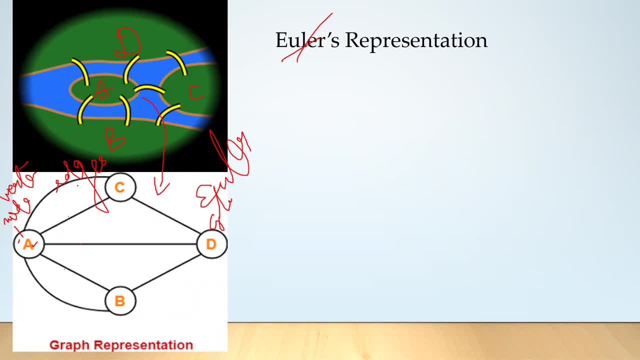 euler cycle know you pass through each and every edge exactly once and then come back to the starting point, Euler's cycle. okay now, if you think logically, now let's come to the solution, let's try giving a solution for this. okay, imagine you have a vertex, or you have a vertex called a. 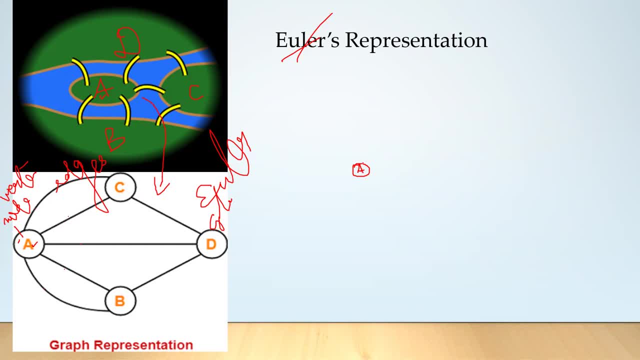 okay, you go out from A. you go out from A. you should be able to come back to A. okay, then only that cycle will be completed. okay, you should be able to go out from A and you should be able to come back to A. now, imagine you are able to go out. 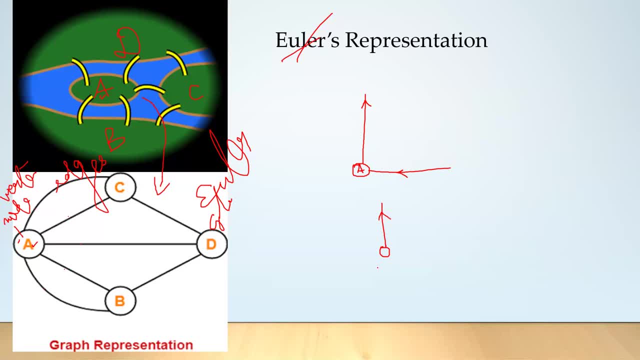 and not come back to A. you should be able to come back to A, not come back to a. you know that cycle will not be completed. so very simple: how many ever times you go out, those many times you should be able to come back, which means the number of edges. 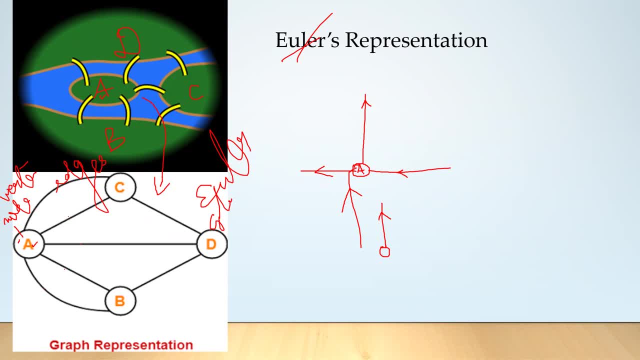 the number of edges from a particular vertex. it should be even. then only you can have a cycle. you can have a cycle only if the number of edges from each vertex is even. imagine you can go out and then you can't come back. you will never have a cycle. your cycle will be incomplete, but you know. 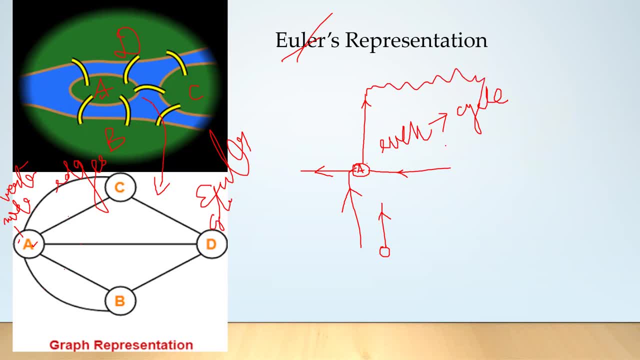 able to go out, and then you know, travel somehow, somehow travel through any number of paths, and all that, and then, if you're able to come back to that particular vertex itself, you can say that you have a cycle. you can have a cycle only if the number of edges from each vertex is even. 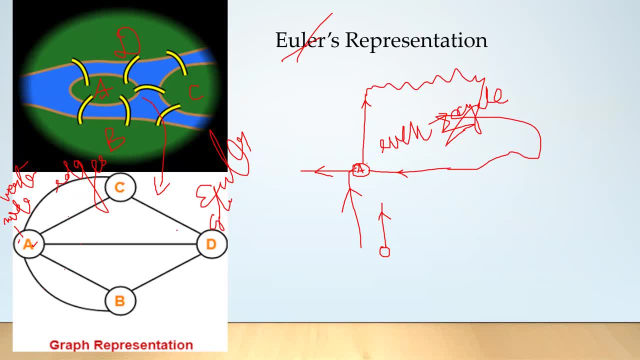 so similarly, each and every vertex over here. if they have even number of edges going out of it, you can have a cycle. we can look here this, look here, let's think about a. you have one, two, three, four, five. there is no possibility of an Euler cycle in this particular graph. if anyone 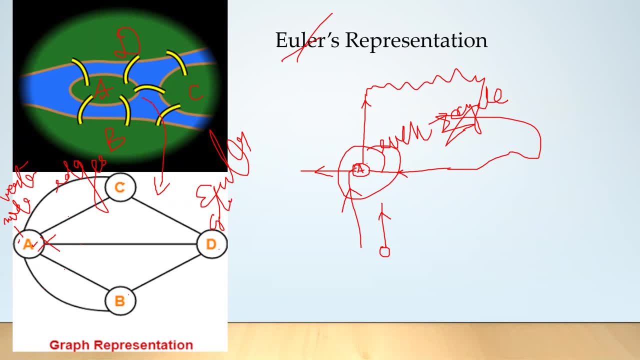 vertex does not have even number of edges, your Euler cycle will not be satisfied. okay, let's look each and everything. one itself dissatisfied, the cycle will not hold. look here: c- dissatisfied, d dissatisfied, d dissatisfied. very simple: you cannot have an Euler cycle, which means this problem. 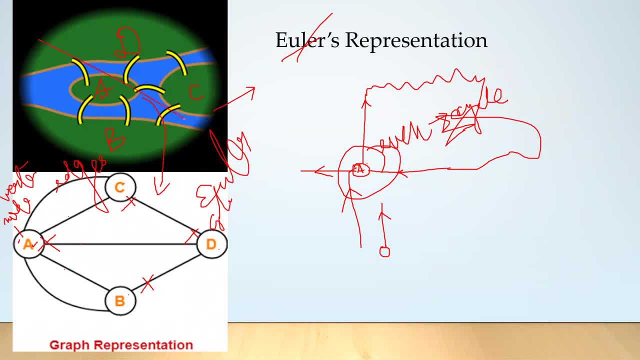 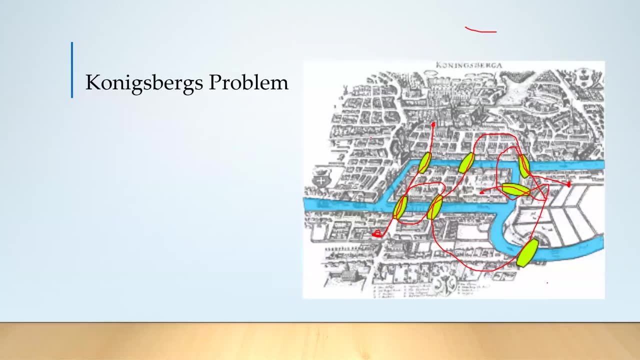 you do not have a solution. there is no solution for this problem. if I go back, okay, this Konigsberg problem, that game which they tried in the 17th century. it has no possible solution. you cannot start from a particular point, you cannot travel through each. 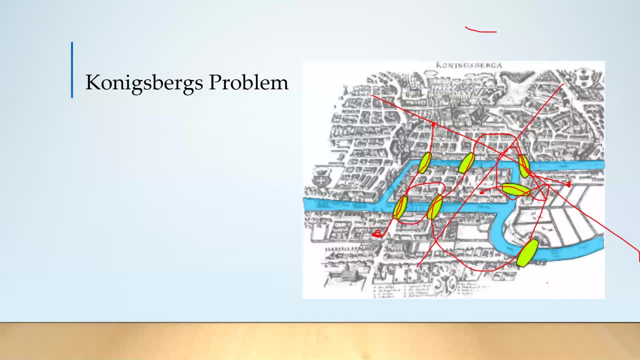 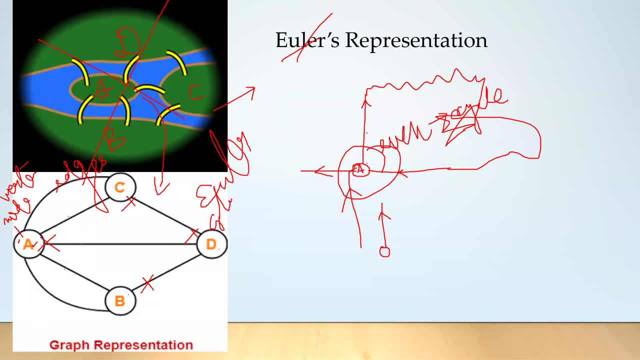 it mathematically. how did he prove it? he proved that you know, if you need to have a cycle, you should have even numbers coming out of it, you should have even number of edges coming out of it. and this particular Konigsberg bridge problem: it does not have even number of. 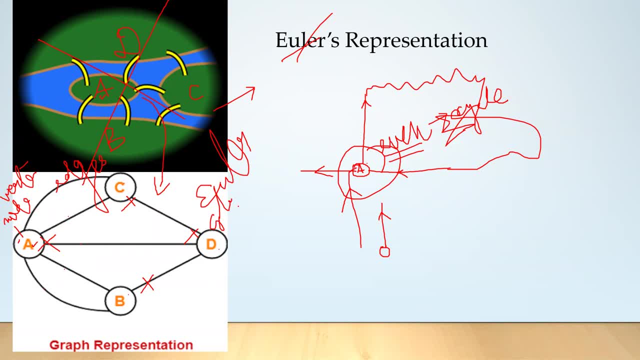 edges coming out of each vertex, which means, you know, it is a problem which has no solution. but interestingly, Euler, he did not tell that this does not have a solution. okay, he did not. sorry, he did not say that I cannot solve the problem. solve the problem. instead, he said: I proved that. 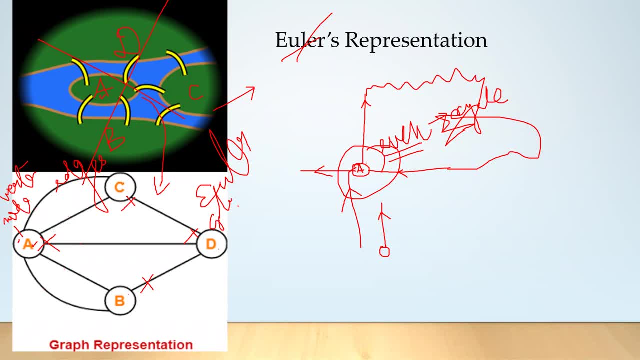 this problem cannot be solved. I proved that this problem cannot be solved. thus this problem is solved. chapter closed. okay, this does not have a solution, correct, but Euler proved it. Euler proved it- that it cannot be solved. thus this problem is solved. so there's no more discussions on this problem. 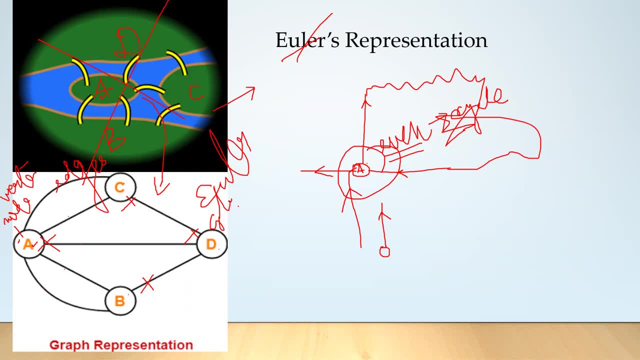 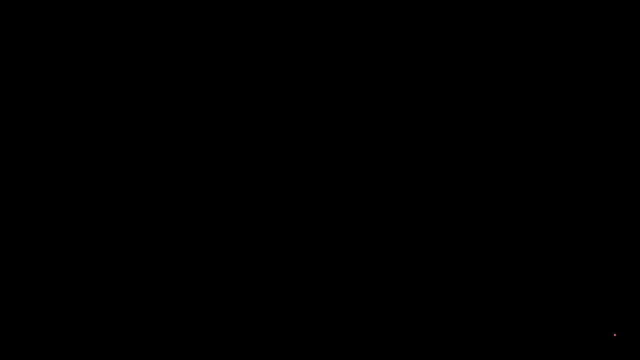 okay, this is a problem which cannot be solved, and I have proved it mathematically that it cannot be solved. therefore, this problem is solved. so this is how Euler came up with a solution for a problem which did not have a solution. so let's come back to the problems in computer science. as I told you, 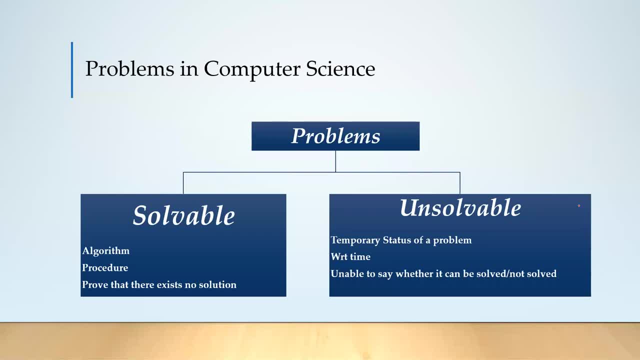 problems in computer science are divided into two. either they are solved or they are not solved. so let's come back to the problems in computer science. either they are solved or they are not solved. so let's come back to the problems in computer science, solvable or unsolvable. solvable problems: as we saw earlier, they will have an algorithm. 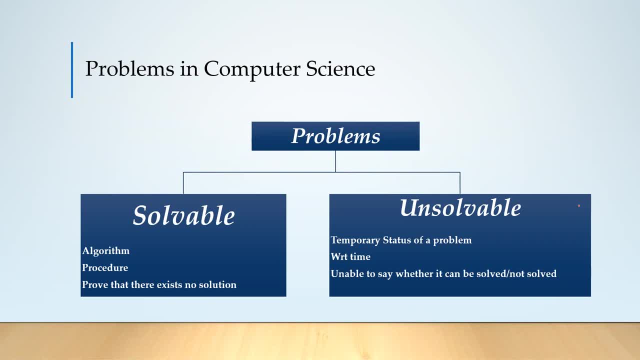 they will have a procedure and not only you get an answer for it. you need not get an. you need not always get an answer for a solvable problem. if you prove that there exists no solution for the problem, that problem, it comes under the category of solvable problem. so let's come back to 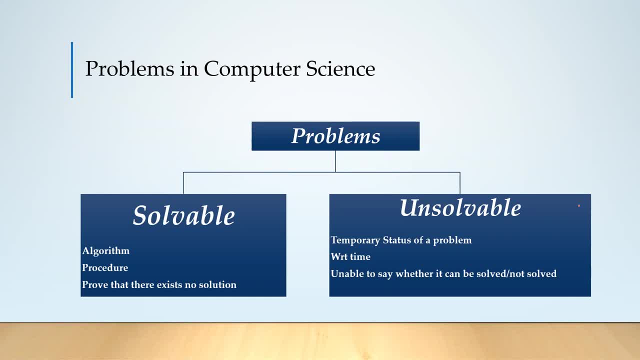 for the problem that problem. it comes under the category of solvable problem. so let's come back to for the problem that problem. it comes under the category of solvable problem. so let's come back to. of a solvable problem example: a conics bug. of a solvable problem example: a conics bug. 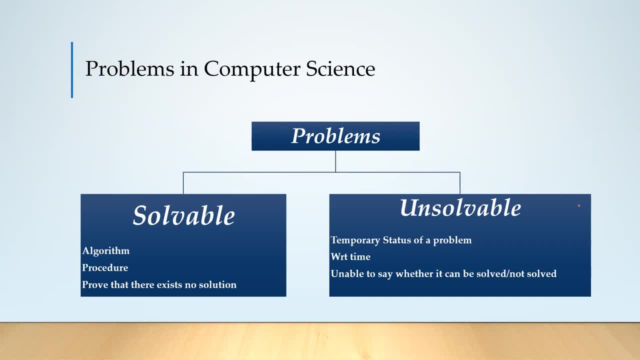 of a solvable problem. example: a conics bug. okay, there is no solution, but it has. okay, there is no solution, but it has. okay, there is no solution, but it has mathematically been proved that there is mathematically been proved that there is mathematically been proved that there is no solution, which means that problem is a. 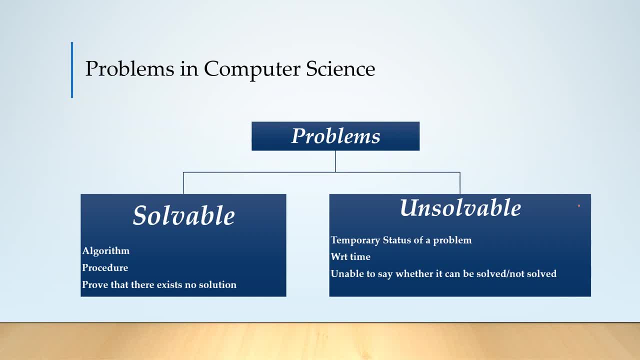 no solution, which means that problem is a no solution, which means that problem is a solvable problem. so solvable problems are solvable problem. so solvable problems are solvable problem. so solvable problems are problems which have an algorithm. they problems which have an algorithm, they. 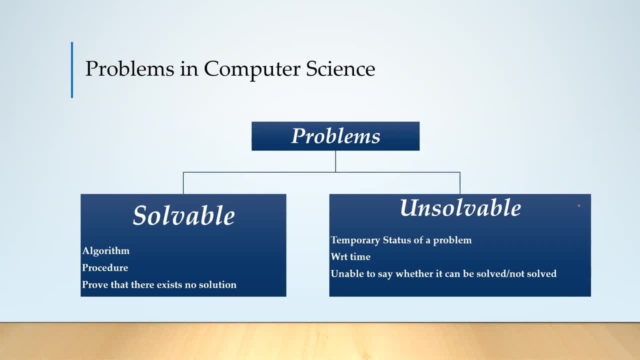 problems which have an algorithm, they will have a procedure, will have a procedure, will have a procedure. or it can be proved that there exists, or it can be proved that there exists, or it can be proved that there exists. no possible solution for such a problem. no possible solution for such a problem. 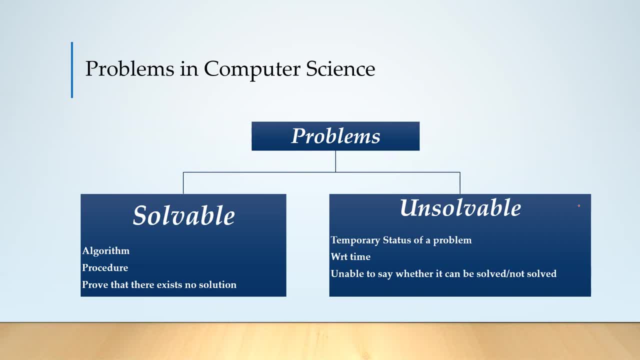 no possible solution for such a problem. similarly, you even have a category called similarly, you even have a category called similarly, you even have a category called unsolvable problems. now unsolvable problems, now unsolvable problems. now this unsolvable problems, this unsolvable problems, this unsolvable problems. you know, you can think of it like this: 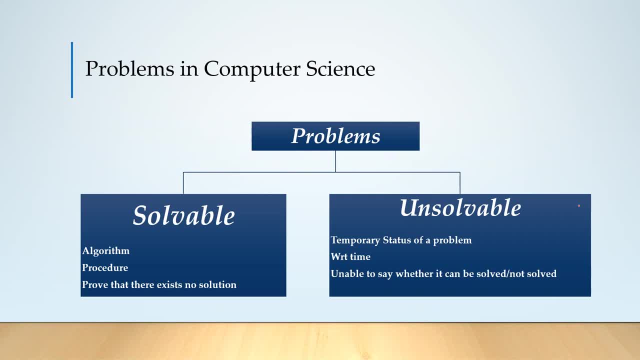 you know you can think of it like this. you know you can think of it like this. imagine some, uh. imagine some. uh imagine some uh. hundred oilers period. hundred oilers period. hundred oilers period, oilers period: nobody would have ever oilers period, nobody would have ever. 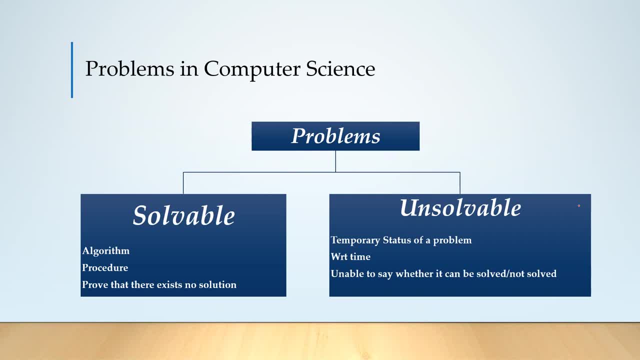 oilers period. nobody would have ever thought of taking online classes. thought of taking online classes, thought of taking online classes, isn't it nobody would have thought of? isn't it nobody would have thought of? isn't it nobody would have thought of? like you know, internet connection. 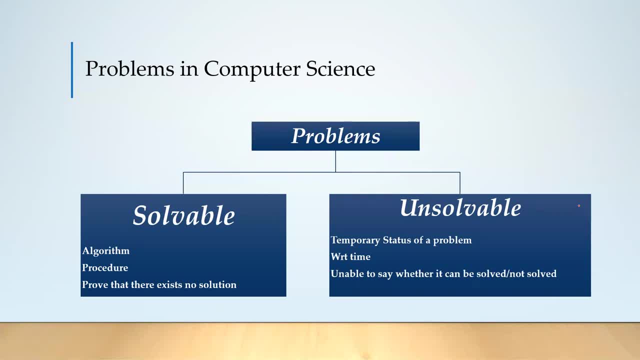 like you know internet connection. like you know internet connection. student sitting at home, the teacher in student sitting at home, the teacher in student sitting at home, the teacher in her home, her home, her home, uh uh, there is uh all this wi-fi and all. uh uh, there is uh all this wi-fi and all. 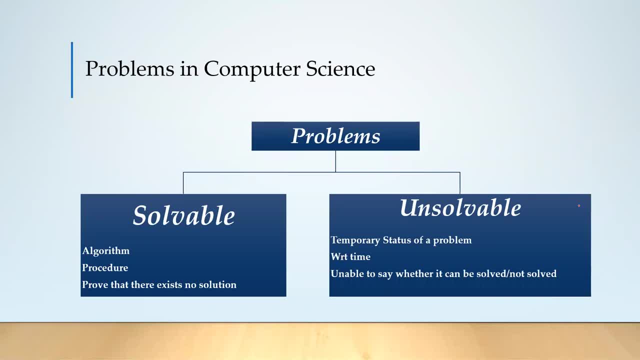 uh, uh. there is uh, all this wi-fi and all that, that, that i share my screen to you 100 years back. i share my screen to you 100 years back. i share my screen to you 100 years back. that was something which people could. that was something which people could. 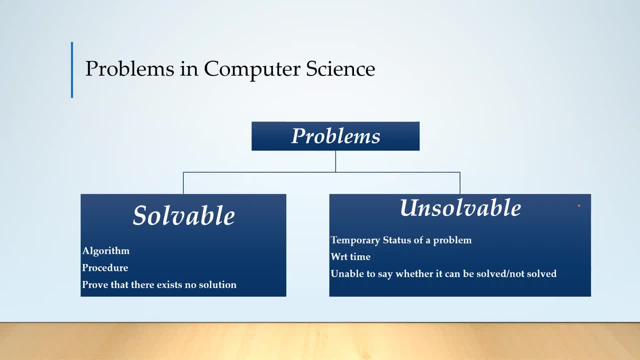 that was something which people could have never have, never have, never thought about. but you know after a thought about, but you know after a thought about, but you know after a period of time. it is very much solvable 100 years. it is very much solvable 100 years. 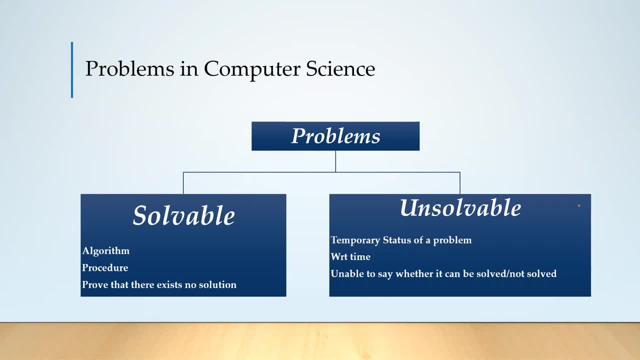 it is very much solvable. 100 years before, before, before my online teaching, it was unsolvable. my online teaching, it was unsolvable. my online teaching, it was unsolvable. but you know, but you know, but you know. 100 years down the line, 2020, the pandemic. 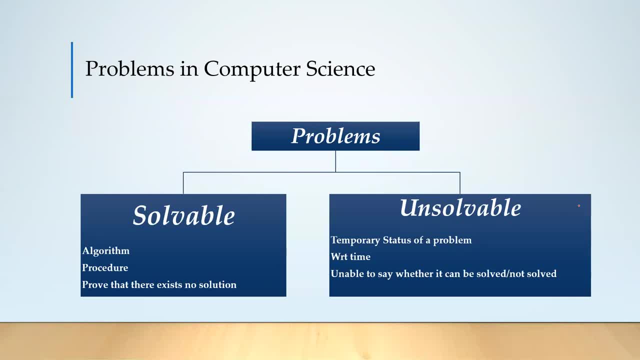 100 years down the line 2020, the pandemic. 100 years down the line 2020, the pandemic. online teaching is very much solvable, so online teaching is very much solvable, so online teaching is very much solvable. so unsolvable problems: they're actually a. 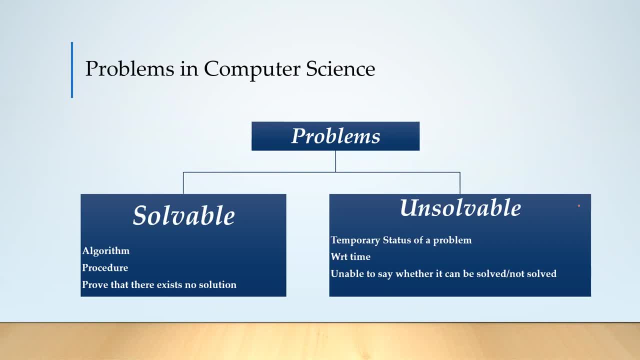 unsolvable problems. they're actually a unsolvable problems. they're actually a temporary status of a problem. temporary status of a problem. temporary status of a problem for the time being. you cannot solve it for the time being. you cannot solve it for the time being. you cannot solve it, but might be after some period of time. 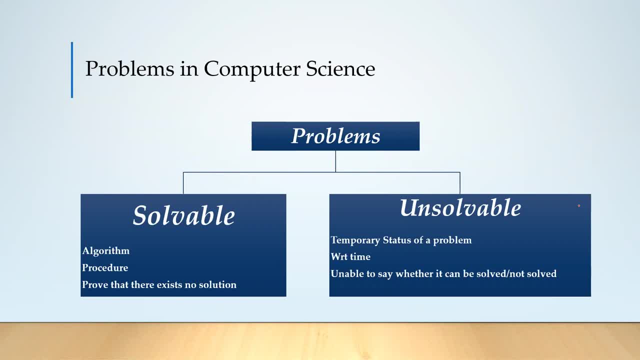 but might be after some period of time. but might be after some period of time. you might be able to solve it, you're not. you might be able to solve it, you're not. you might be able to solve it. you're not sure, sure, sure, you are not sure you might solve it. you. 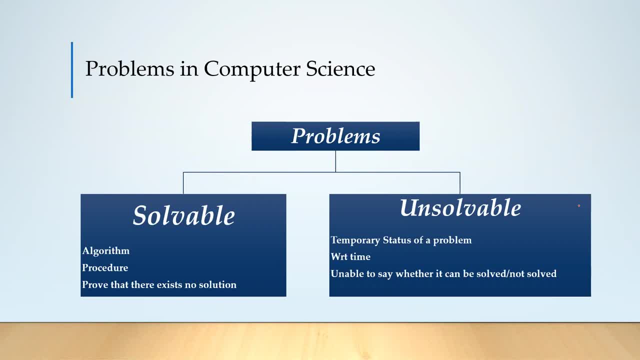 you are not sure you might solve it. you, you are not sure you might solve it. you might not solve it, might not solve it. but you know, as of now, with respect to, might not solve it. but you know, as of now, with respect to, might not solve it. but you know, as of now, with respect to time when i clap my hands, you cannot. 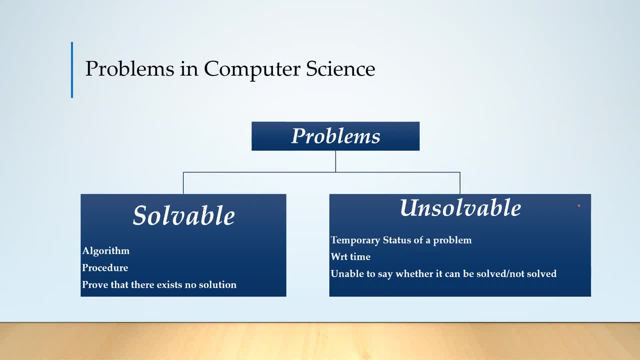 time when i clap my hands, you cannot time. when i clap my hands, you cannot disappear, disappear, disappear with respect to time. you know i cannot uh with respect to time. you know i cannot uh with respect to time. you know i cannot uh count the stars in the sky. 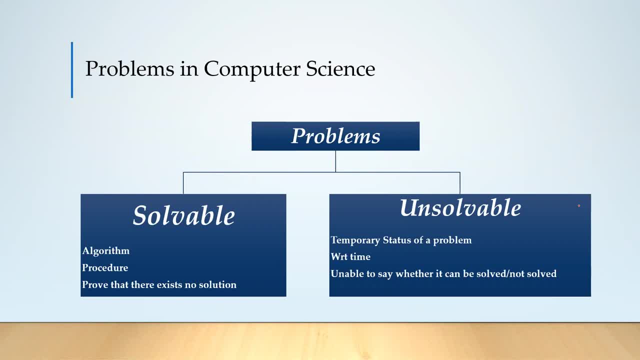 count the stars in the sky. count the stars in the sky. you know, division by zero. i cannot do all. you know division by zero. i cannot do all. you know division by zero. i cannot do all that. that. that okay. so your okay. so your okay. so your category of unsolvable problems they are: 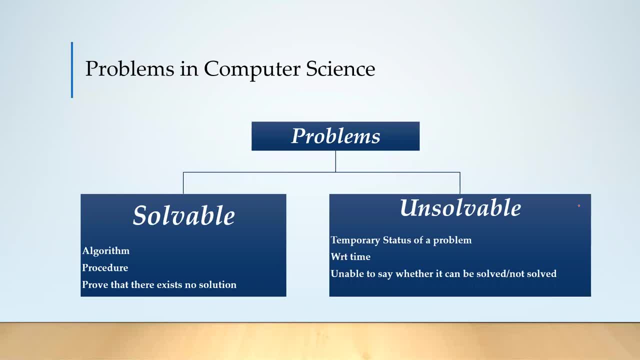 category of unsolvable problems. they are category of unsolvable problems. they are actually the set of problems, actually the set of problems, actually the set of problems which which which, for the time being, they cannot be solved, for the time being, they cannot be solved, for the time being they cannot be solved, and you know. 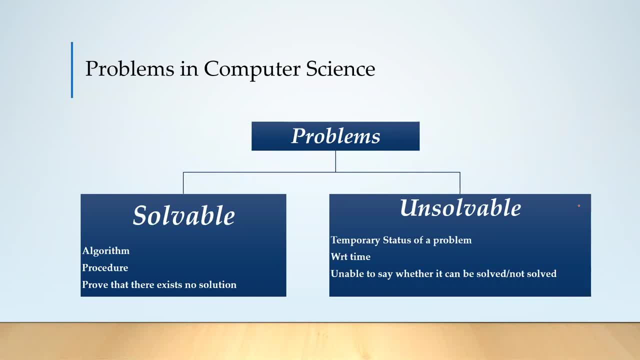 and you know, and you know whether it can be solved or cannot be, whether it can be solved or cannot be, whether it can be solved or cannot be solved, only time can tell solved, only time can tell. so those are the categories of unsolvable. so those are the categories of unsolvable. 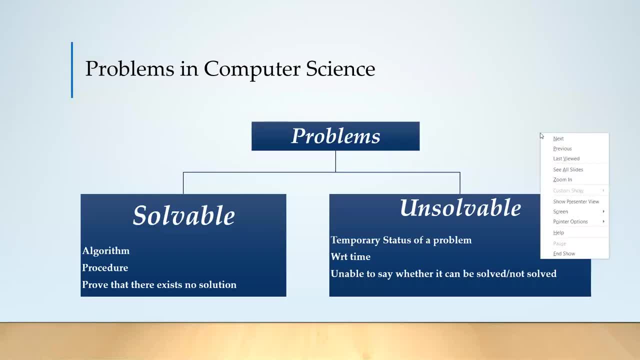 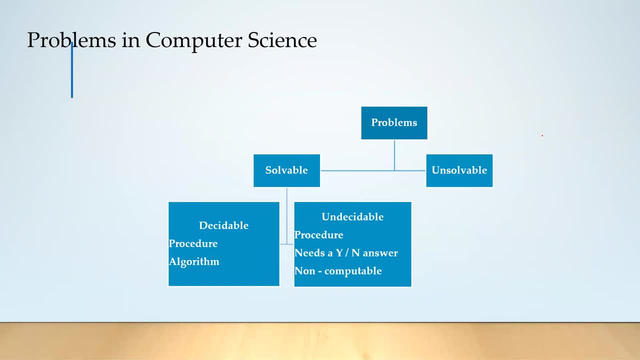 so those are the categories of unsolvable problems, now solvable problems. they are now solvable problems. they are now solvable problems. they are in two categories. you call them in two categories. you call them in two categories. you call them decidable and undecidable. 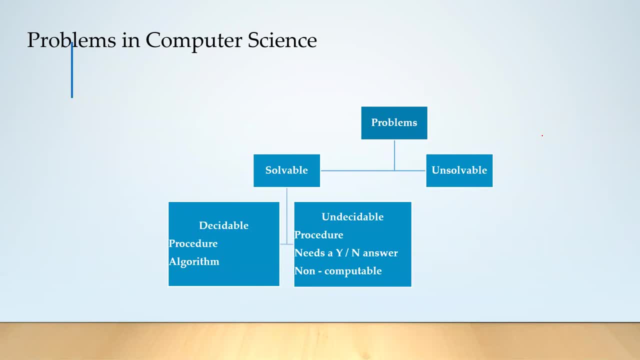 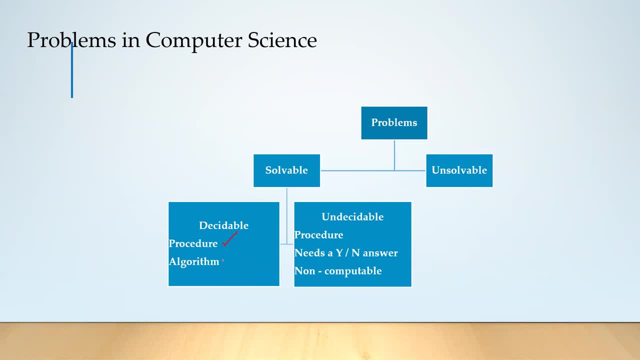 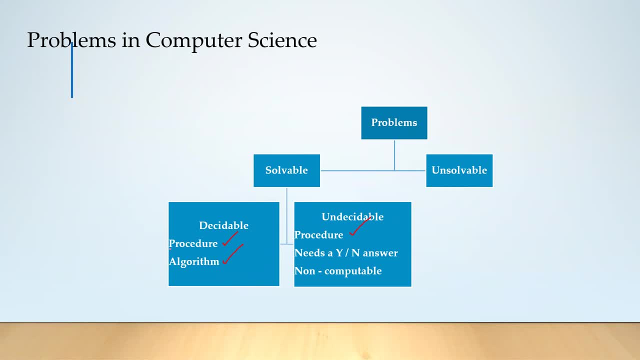 but they will not have a, but they will not have a problem. so before we go detail into problem, so before we go detail into problem, so before we go detail into that, let me just give you a small idea that. let me just give you a small idea. 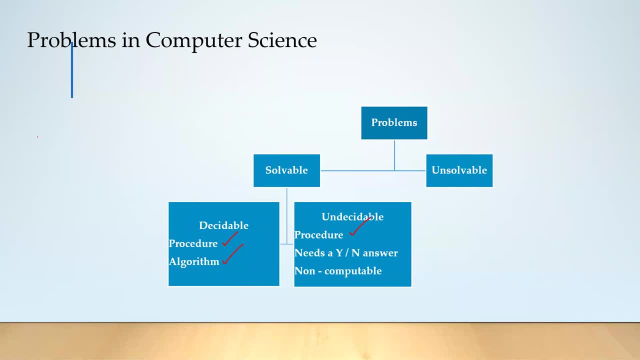 that let me just give you a small idea about, about, about. what is the difference between a? what is the difference between a? what is the difference between a procedure and an algorithm? imagine you procedure and an algorithm. imagine you procedure and an algorithm. imagine you want to calculate. 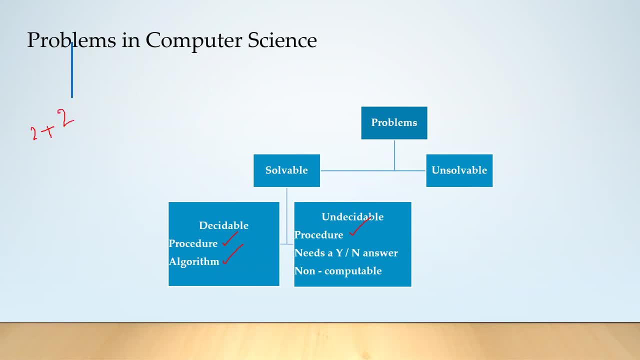 want to calculate, want to calculate two plus two. you want to calculate two, two plus two. you want to calculate two plus two. sum of two numbers plus two. sum of two numbers plus two. sum of two numbers. okay, procedure is get a number. okay procedure is get a number. 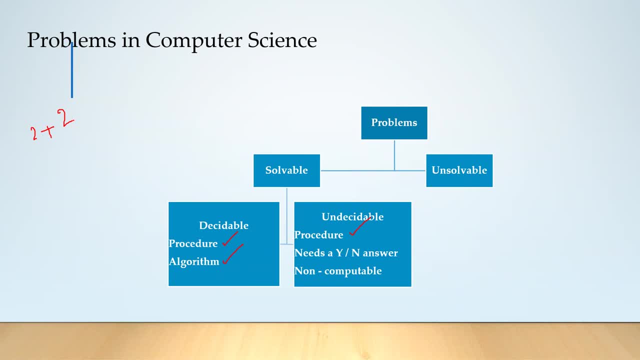 okay procedure is: get a number, get another number, add it up the result. get another number, add it up the result. get another number, add it up the result. that's the procedure. okay, you have a. that's the procedure. okay, you have a. that's the procedure. okay, you have a methodology. procedure is nothing but a. 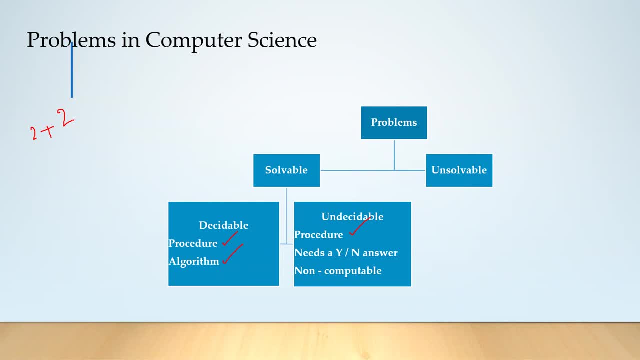 methodology procedure is nothing but a methodology procedure is nothing but a methodology: step by step process methodology. step by step process methodology, step by step process. if you have a step by step process to, if you have a step by step process to, if you have a step by step process to do it. 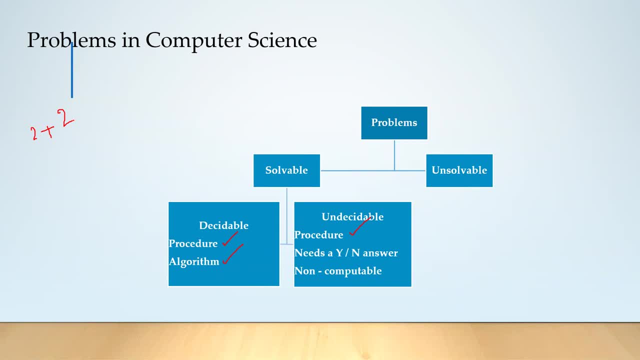 do it, do it. it can either be decidable or it can either be decidable or it can either be decidable or undecidable. algorithm means algorithm means. algorithm means a procedure, it becomes an algorithm. if a procedure, it becomes an algorithm. if a procedure, it becomes an algorithm. if i know, 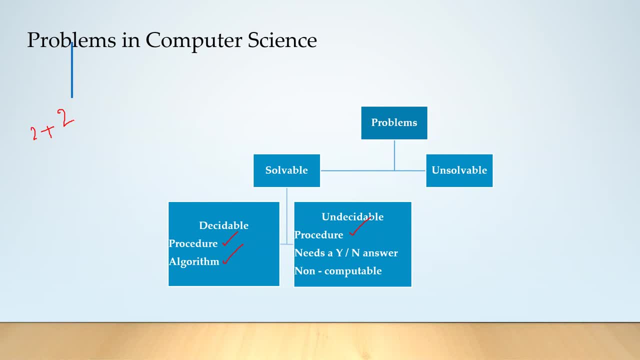 i know, i know the approximate time needed to do it. the approximate time needed to do it, the approximate time needed to do it- two plus two, two plus two, two plus two. i i know what time is needed. i, i know what time is needed. i, i know what time is needed. okay, now, if i know the procedure and i. 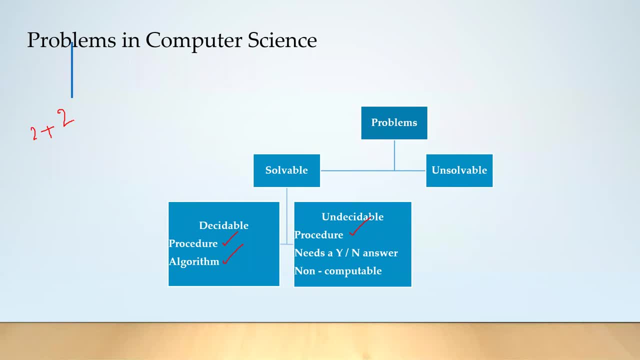 okay now, if i know the procedure and i. okay now, if i know the procedure and i, if i even have an algorithm, if i'm able, if i even have an algorithm, if i'm able, if i even have an algorithm, if i'm able to calculate the approximate time. 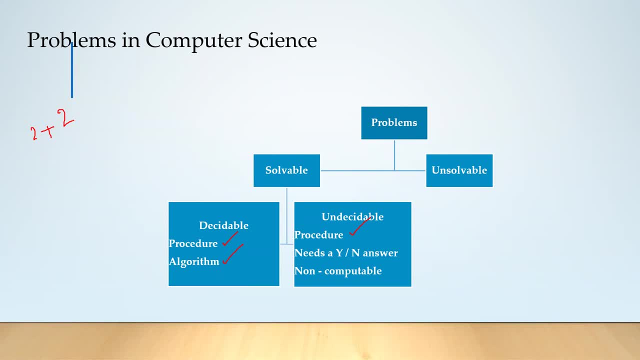 to calculate the approximate time. to calculate the approximate time, i say the problem is a decidable. i say the problem is a decidable. i say the problem is a decidable problem. let's say you're sorting n problem. let's say you're sorting n problem. let's say you're sorting n numbers. you're doing a bubble sort. 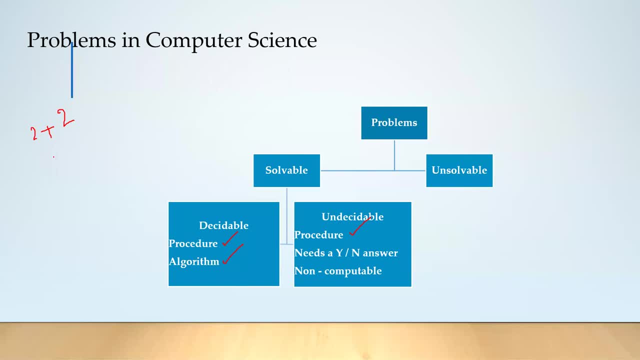 numbers: you're doing a bubble sort. numbers: you're doing a bubble sort. imagine you're doing a bubble sort. you imagine you're doing a bubble sort. you imagine you're doing a bubble sort. you know how to do a bubble sort. know how to do a bubble sort. 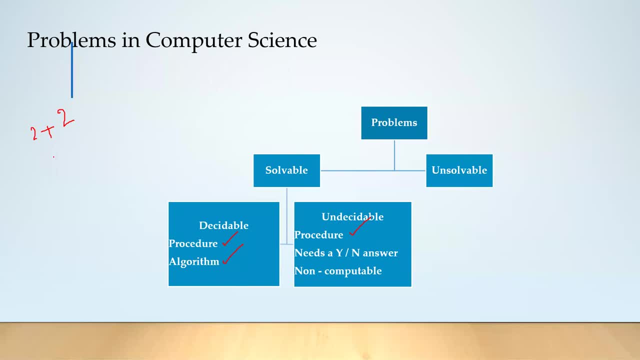 know how to do a bubble sort step by step. you know how to do it. get step by step. you know how to do it get step by step. you know how to do it. get n numbers. do the bubbling and all that. n numbers, do the bubbling and all that. 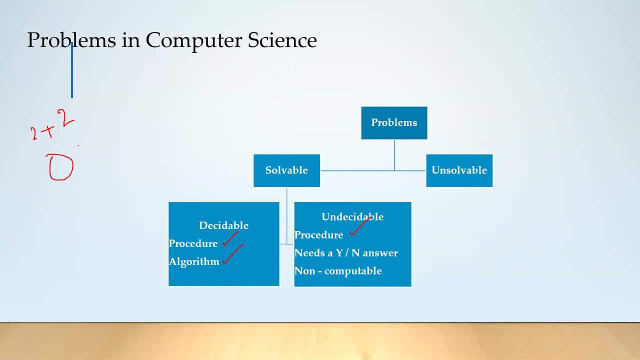 n numbers, do the bubbling and all that. you know the procedure. you even have an. you know the procedure. you even have an. you know the procedure. you even have an algorithm. you are able to calculate algorithm. you are able to calculate algorithm. you are able to calculate, let's say, bubble sort. you have a. 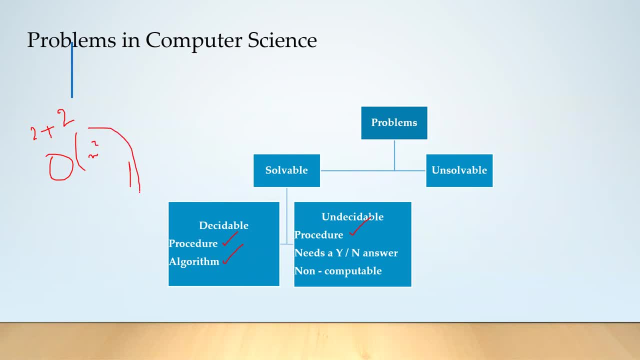 let's say, bubble sort. you have a, let's say bubble sort. you have a complexity of o and square. complexity of o and square, complexity of o and square. yeah, yeah, yeah, you have an algorithm. you have an algorithm. you have an algorithm. okay, you can find out how much time is. 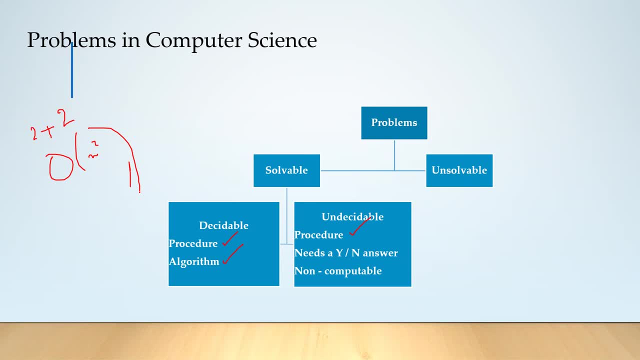 okay. you can find out how much time is okay. you can find out how much time is needed, needed, needed. you can find out how much time is needed. you can find out how much time is needed. you can find out how much time is needed. it comes under the category of a. 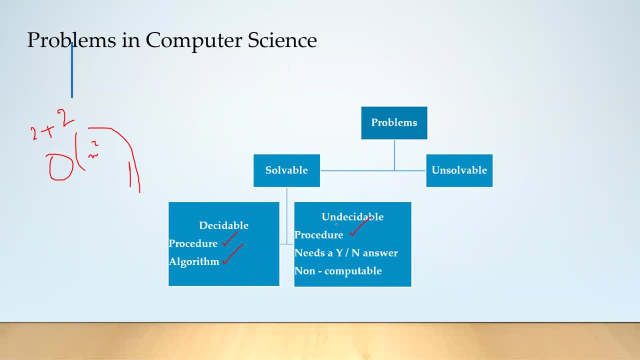 it comes under the category of a. it comes under the category of a decidable problem. decidable problem, decidable problem. undecidable problem means you know how undecidable problem means. you know how undecidable problem means, you know how to do it, to do it. 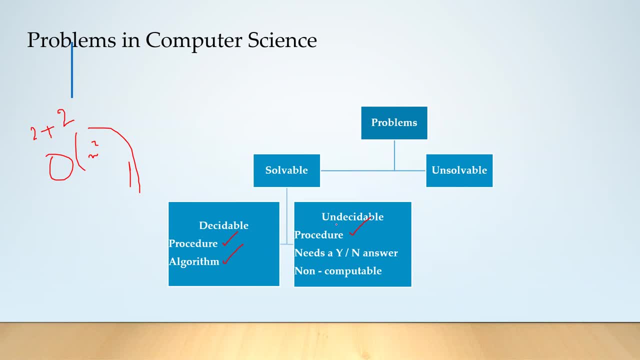 to do it. you know how to do it, but you know how to do it. but you know how to do it, but you do not know how much. you do not know how much. you do not know how much time it will take. time it will take, time it will take. you do not know how much time that. 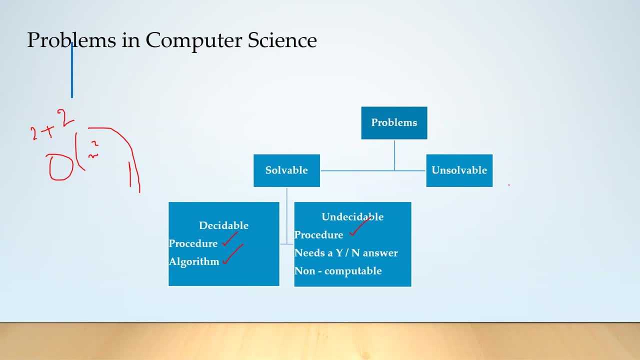 you do not know how much time that. you do not know how much time that particular thing will take. let's say particular thing will take. let's say particular thing will take. let's say imagine, imagine. imagine. imagine you're having a placement drive. imagine you're having a placement drive. 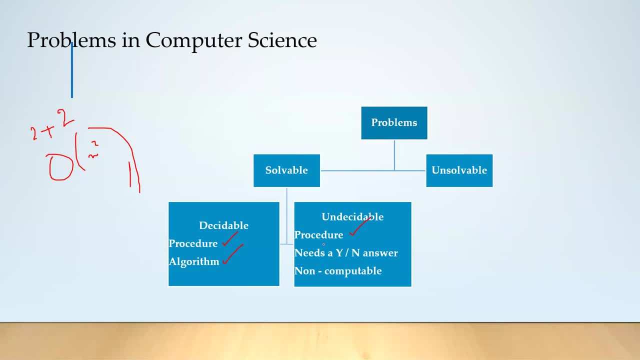 imagine you're having a placement drive. you have all these uh colleges coming in. you have all these uh colleges coming in. you have all these uh colleges coming in. you have all these n number of colleges. you have all these n number of colleges. you have all these n number of colleges coming in. 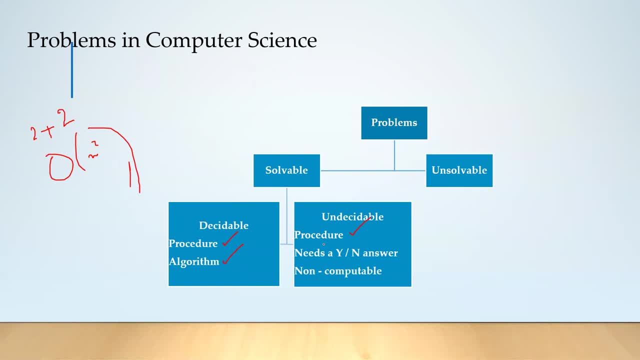 coming in, coming in and infosys, they are giving a common and infosys, they are giving a common and infosys, they are giving a common campus recruitment, a technical test, a campus recruitment, a technical test, a campus recruitment, a technical test, a technical test for everybody and all of 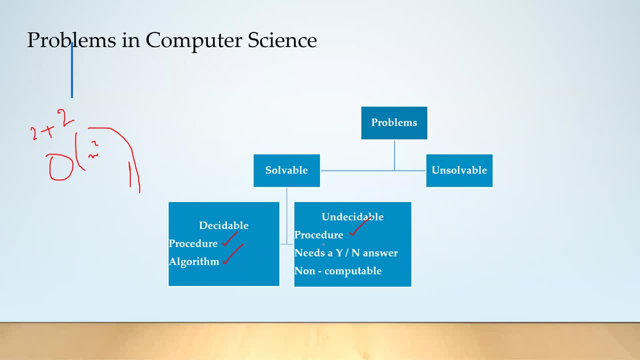 technical test for everybody and all of technical test for everybody, and all of you are appearing for the test. you are appearing for the test. you are appearing for the test. okay, and imagine, okay, and imagine, okay and imagine. the question is: the question is. the question is: you want to become? 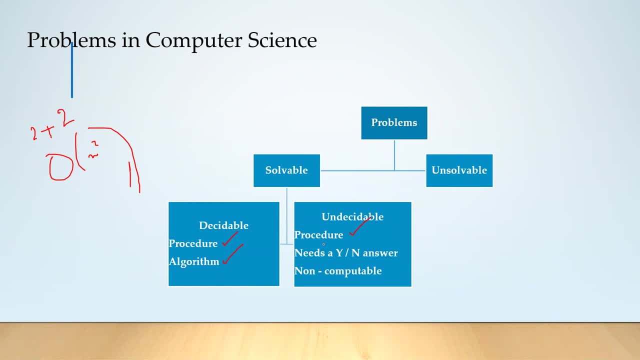 you want to become. you want to become number one in that infosys test, number one in that infosys test, number one in that infosys test. okay, you want to become all the colleges. okay, you want to become all the colleges. okay, you want to become all the colleges. they are giving a placement drive, or 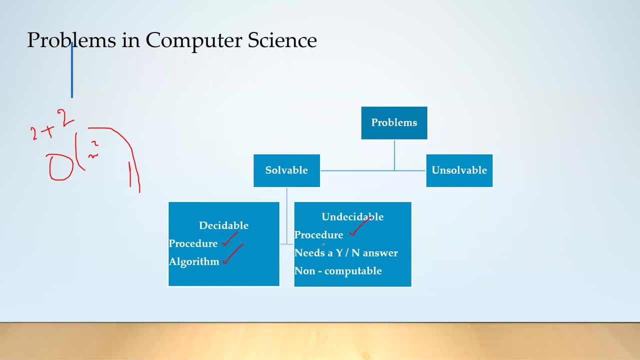 they are giving a placement drive, or they are giving a placement drive, or there are thousand number of students. there are thousand number of students. there are thousand number of students. writing it, writing it, writing it. you want to become number one in that. you want to become number one in that. 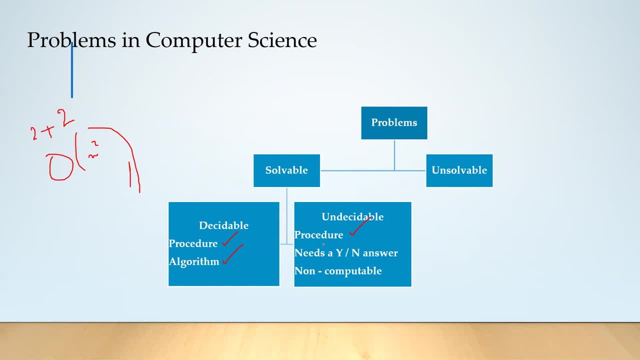 you want to become number one in that test, test, test. okay. so what all should you be doing? okay? so what all should you be doing? okay? so what all should you be doing? let's say you have to do preparation you. let's say you have to do preparation you. 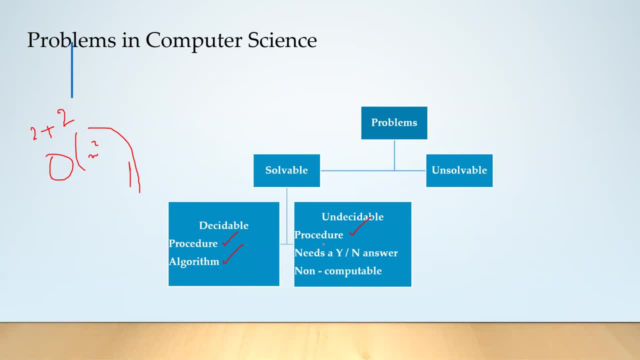 let's say, you have to do preparation. you have to go on doing a lot of mocks, have to go on doing a lot of mocks, have to go on doing a lot of mocks. you have to learn your subjects, okay, you. you have to learn your subjects, okay you. 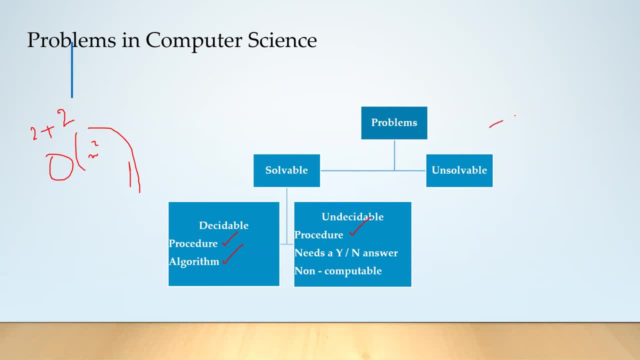 you have to learn your subjects. okay, you know the procedure, know the procedure. know the procedure. okay, you know the procedure. how to clear. okay, you know the procedure how to clear. okay, you know the procedure: how to clear reinforces, reinforces, reinforces. you know the procedure, you know the. 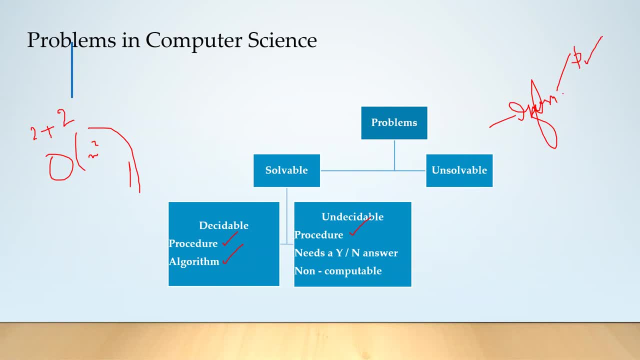 you know the procedure, you know the, you know the procedure, you know the procedure, procedure, procedure. you very well know how to do it step by you very well know how to do it step by you very well know how to do it step by step, step, step. but are you exactly? 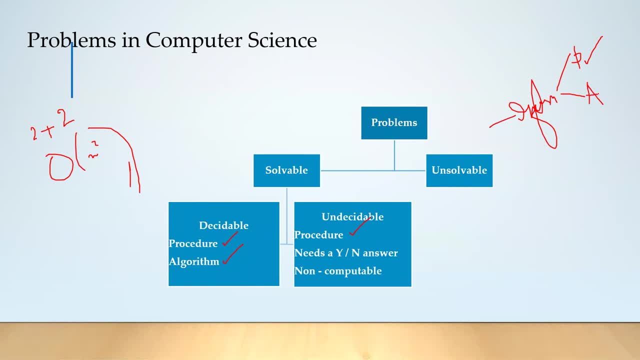 but are you exactly? but are you exactly able to tell me within what period? will able to tell me within what period will able to tell me within what period will you become number one? you become number one. you become number one. first attempt, you might not be number. 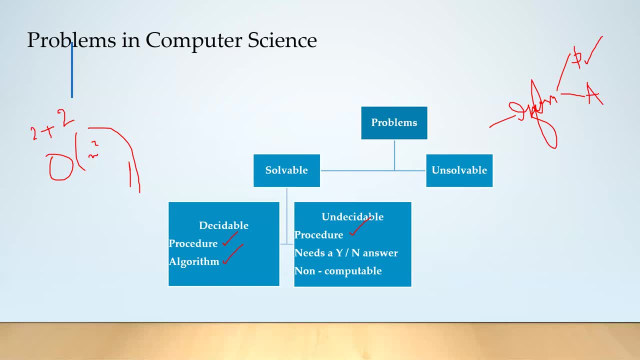 first attempt. you might not be number first attempt, you might not be number one. second attempt, one second attempt, one second attempt. you might not be number one, you, you, you might not be number one, you, you, you might not be number one, you, you, exactly. you cannot tell the time. 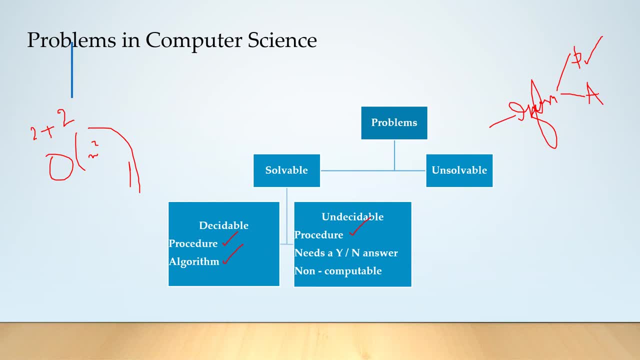 exactly. you cannot tell the time exactly. you cannot tell the time. if you're lucky enough, you can be first. if you're lucky enough, you can be first. if you're lucky enough, you can be first time time time. okay, if you are a bit more unlucky, you. 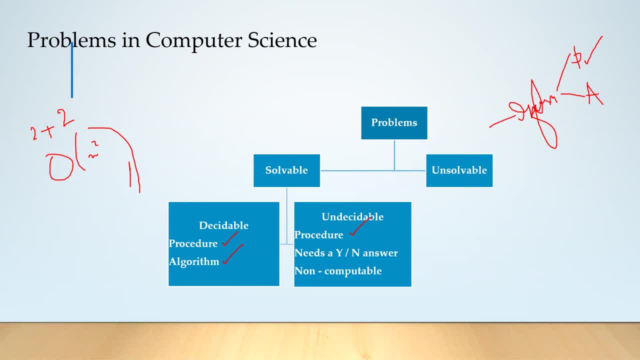 okay if you are a bit more unlucky, you okay, if you are a bit more unlucky, you might be third time, but you know my might be third time, but you know my might be third time, but you know my question is: you should be number one in question? is you should be number one in? 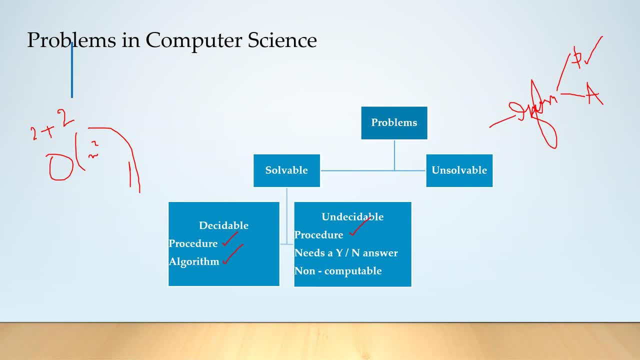 question is: you should be number one in kerala writing the enforcers exam. kerala- writing the enforcers exam- kerala- writing the enforcers exam. okay, that is a bit difficult. you cannot. okay, that is a bit difficult. you cannot. okay, that is a bit difficult. you cannot tell that. 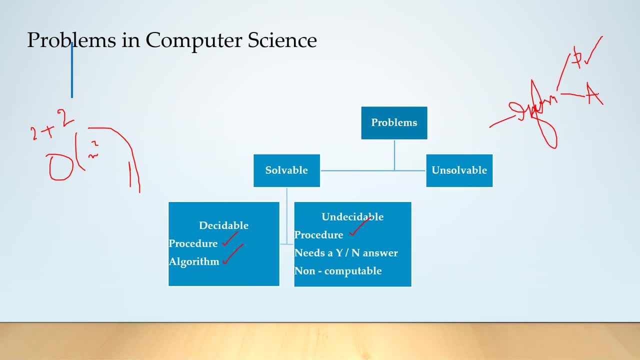 tell that, tell that you might always qualify for the. you might always qualify for the. you might always qualify for the enforcers exam. but becoming number one enforcers exam, but becoming number one enforcers exam, but becoming number one, that is my question. that is my question. 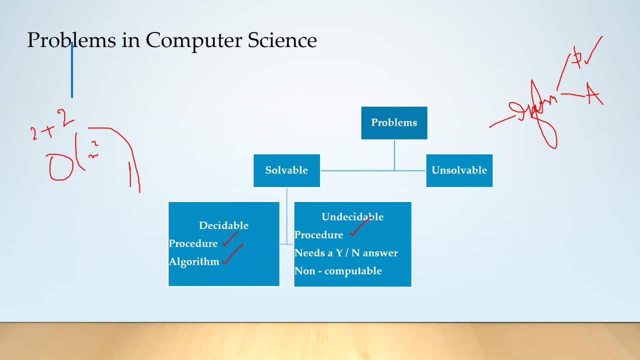 that is my question. you exactly cannot tell me a time in. you exactly cannot tell me a time in. you exactly cannot tell me a time in which, which which you can become number one. so i say an, you can become number one. so i say an, you can become number one. so i say an algorithm for that. 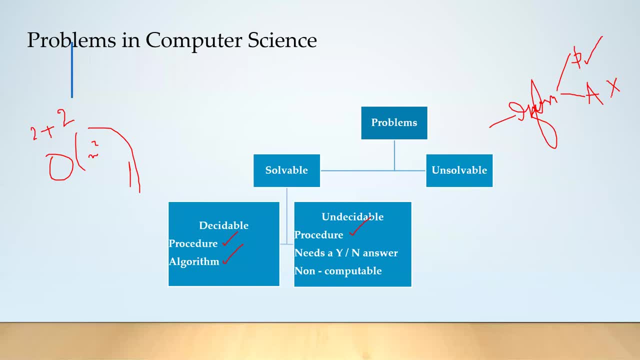 algorithm for that, algorithm for that does not exist, okay, does not exist, okay, does not exist. okay, getting into enforcers: yeah, that will getting into enforcers, yeah, that will getting into enforcers. yeah, that will happen, happen, happen. but becoming the number one, becoming the 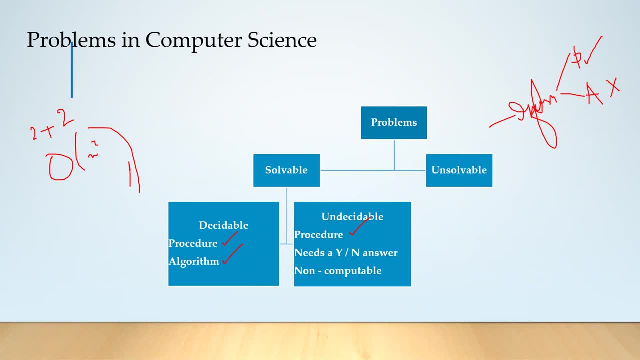 but becoming the number one, becoming the. but becoming the number one, becoming the number one rank in enforcers. i say number one rank in enforcers. i say number one rank in enforcers. i say an algorithm does not exist for it. a. an algorithm does not exist for it, a. 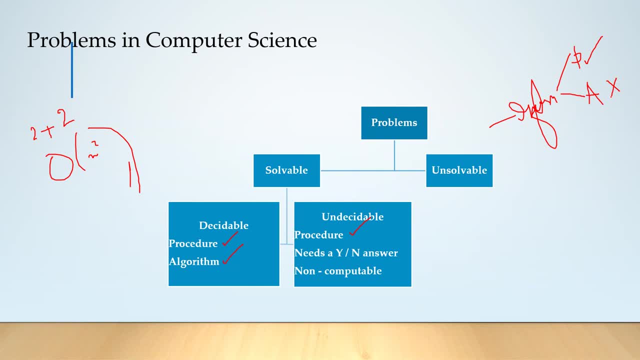 an algorithm does not exist for it. a procedure exists, procedure exists, procedure exists, algorithm doesn't exist. you do not have. algorithm doesn't exist. you do not have, algorithm doesn't exist. you do not have a time frame, a time frame, a time frame. you say it is an undecidable problem. 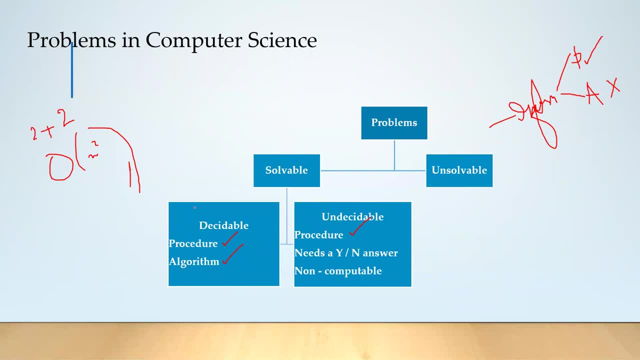 you say it is an undecidable problem. you say it is an undecidable problem getting into enforcers. getting into enforcers, getting into enforcers, yeah, that is possible, yeah, that is possible, yeah, that is possible, but you know, but you know. 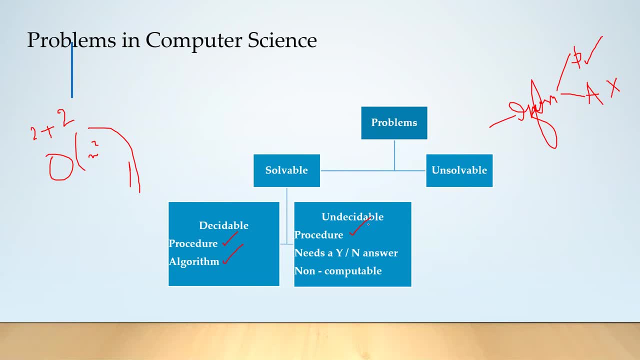 but you know, getting the number one rank in getting the number one rank, in getting the number one rank in enforcers, because i don't have an enforcers, because i don't have an enforcers because i don't have an chief minister of india. 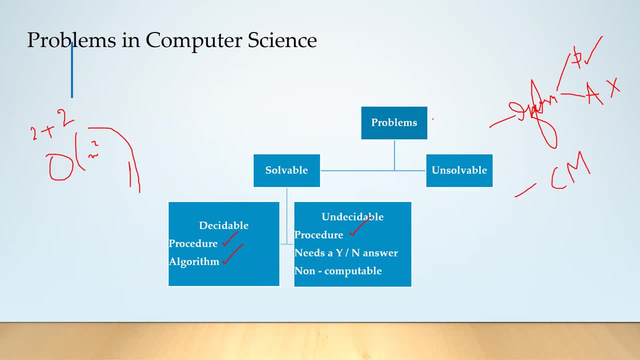 chief minister of india. chief minister of india, you want to become the chief minister of. you want to become the chief minister of. you want to become the chief minister of- sorry chief minister of kerala, sorry chief minister of kerala, sorry chief minister of kerala. okay, you know what to do. you know what. 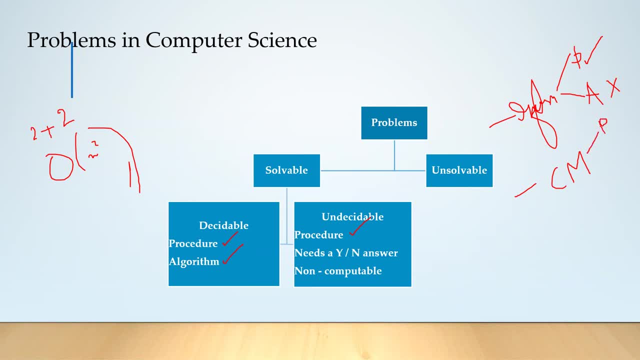 okay, you know what to do. you know what- okay, you know what to do. you know what to do. you should go into uh to do. you should go into uh to do. you should go into uh, some, uh, some, uh, some, uh. you know you should be publicly a known. you know you should be publicly a known. you know you should be publicly a known figure. you should have a bit of politics figure. you should have a bit of politics figure. you should be publicly a known figure. you should have a bit of politics xyz, or you do a lot of. 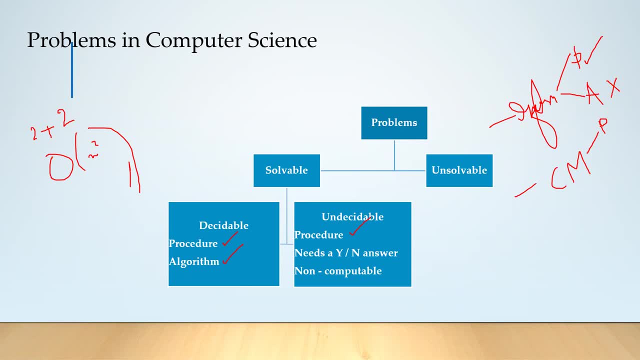 xyz, or you do a lot of xyz, or you do a lot of social work. you get to know with a lot social work, you get to know with a lot social work. you get to know with a lot about people and all that you about people and all that you. 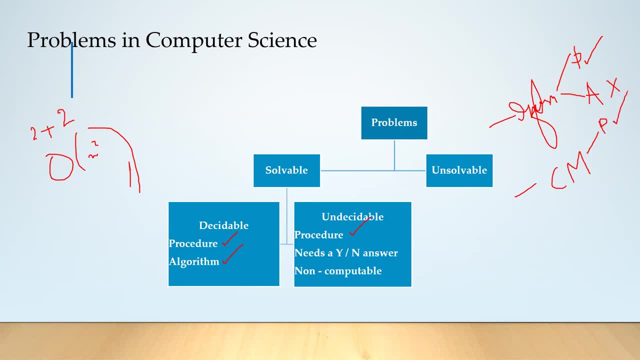 about people and all that. you, you are engaged in their matters. you, you are engaged in their matters. you, you are engaged in their matters. you very well know the procedure, how to get- very well know the procedure, how to get. very well know the procedure, how to get it, but can you tell me a time frame? can? 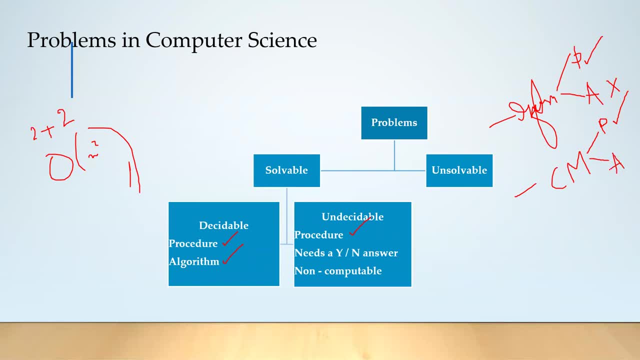 it, but can you tell me a time frame? can it, but can you tell me a time frame? can you tell me within you? tell me within you? tell me, within five years will you be able to become five years? will you be able to become five years? will you be able to become the chief minister, or might be within 20? 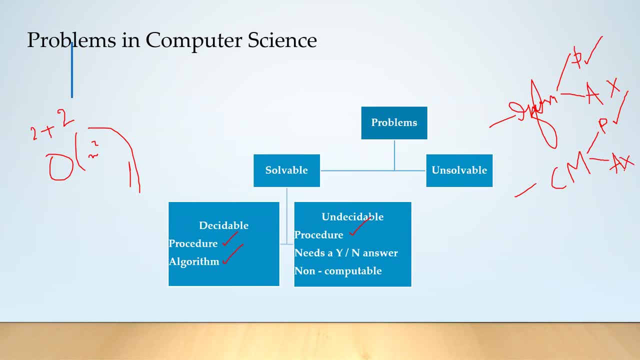 the chief minister, or might be, within 20, the chief minister, or might be within 20 years. will you be able to become the years? will you be able to become the years? will you be able to become the chief minister, chief minister, chief minister, you cannot tell me a time. you cannot. 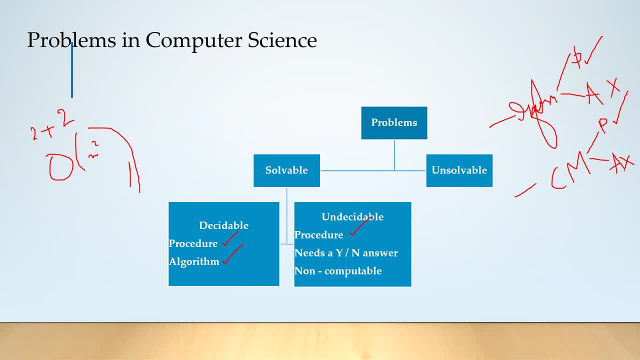 you cannot tell me a time. you cannot. you cannot tell me a time. you cannot tell me a time limit for it. tell me a time limit for it. tell me a time limit for it. so it is an undecidable problem. okay, so it is an undecidable problem, okay. 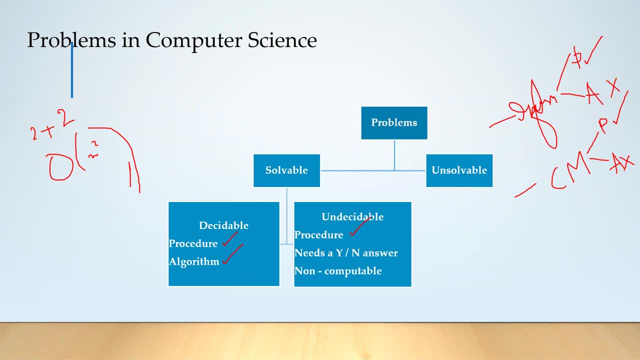 so it is an undecidable problem. okay, almost all the mathematical problems, almost all the mathematical problems, almost all the mathematical problems. they become under decidable, like, like they become under decidable, like, like they become under decidable, like, like, just imagine, just imagine, just imagine. uh, you are thinking about a spanning. 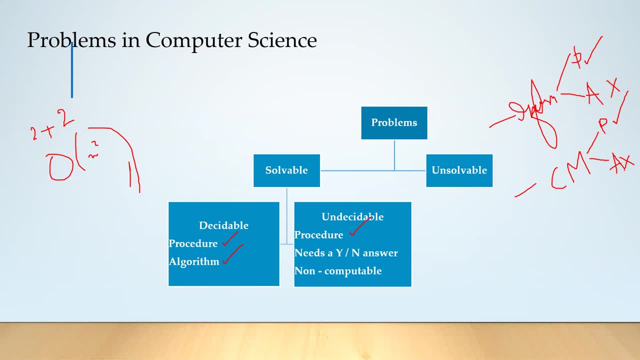 uh, you are thinking about a spanning. uh, you are thinking about a spanning tree. minimum spanning tree tree. minimum spanning tree tree. minimum spanning tree. okay, find the minimum spanning tree. you okay, find the minimum spanning tree. you okay, find the minimum spanning tree. you are given a tree. 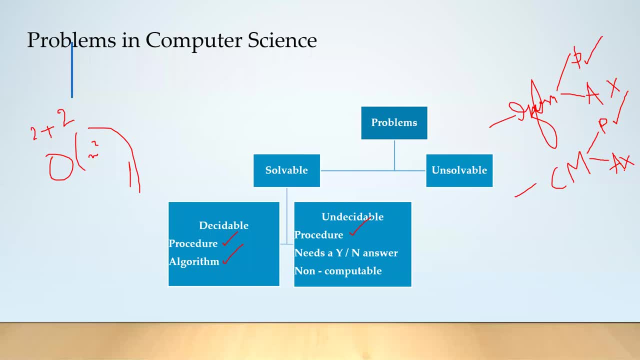 are given a tree, are given a tree, find the minimum spanning tree, you know. find the minimum spanning tree, you know. find the minimum spanning tree. you know that that that ding dong bell, three steps finished. you ding dong bell, three steps finished. you ding dong bell, three steps finished. you will be able to find the minimum. 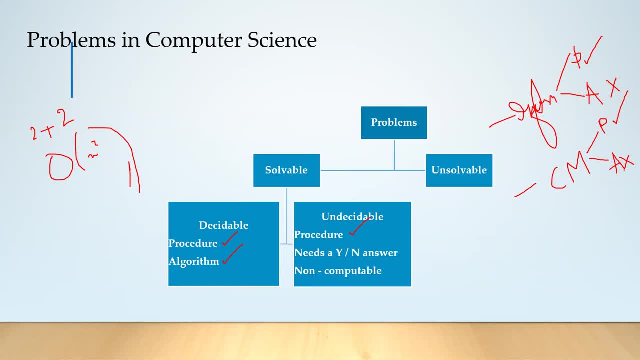 will be able to find the minimum, will be able to find the minimum. spanning tree. you exactly know within spanning tree. you exactly know within spanning tree. you exactly know within three steps you will be able to find out three steps. you will be able to find out three steps. you will be able to find out. you have a formula for that. you have to. 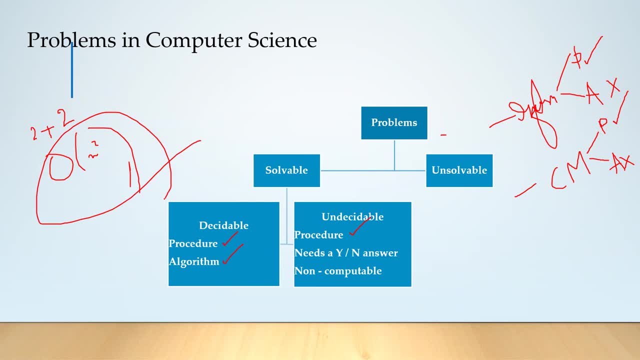 you have a formula for that. you have to. you have a formula for that you have to. you have a formula which will tell you. you have a formula which will tell you. you have a formula which will tell you the time, the time, the time all such problems come under decidable. 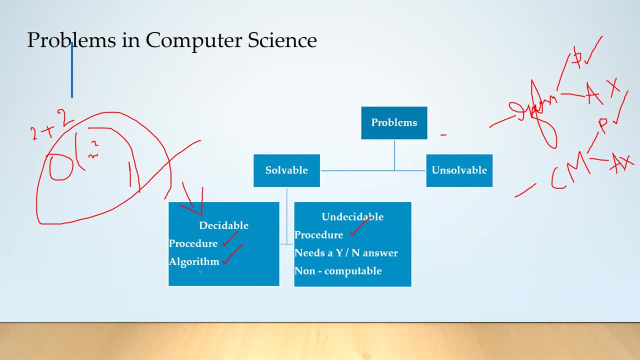 all such problems come under decidable. all such problems come under decidable problems. problems, problems when you have a procedure and when you are when you have a procedure and when you are when you have a procedure and when you are able to tell, able to tell, able to tell the time frame in which you will be able. 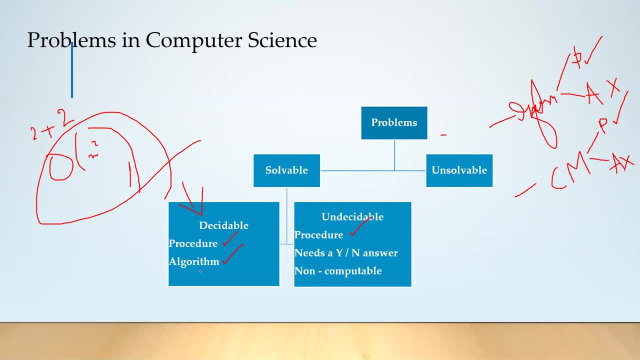 the time frame in which you will be able, the time frame in which you will be able to achieve it approximate, not the exact. to achieve it. approximate, not the exact. to achieve it. approximate, not the exact. approximate time frame. approximate time frame, approximate time frame. you say it is a decidable problem. 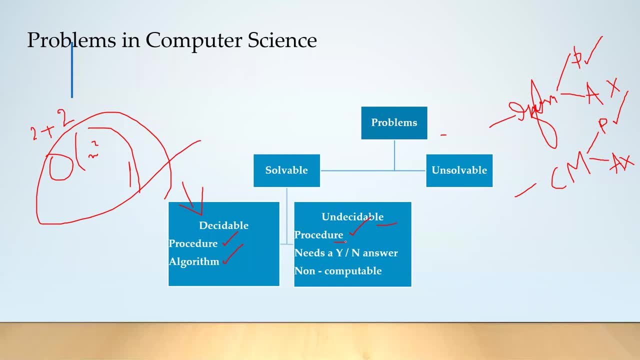 you say it is a decidable problem, undecidable problem. when you only have undecidable problem, when you only have undecidable problem, when you only have a procedure, a procedure, a procedure. you do not have an algorithm, you do not have an algorithm, you do not have an algorithm. okay, and then you need to get an answer. 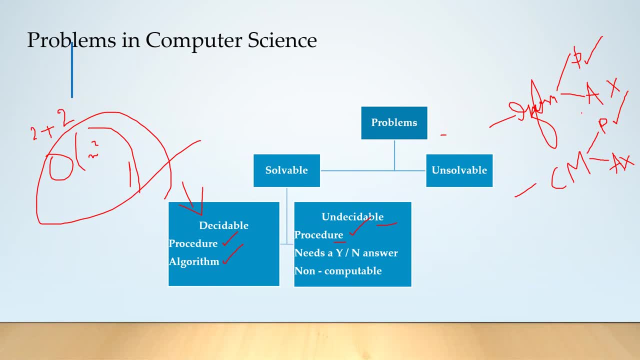 okay, and then you need to get an answer. okay, and then you need to get an answer. like you know, like you know, like you know, will you be able to achieve impulses in? will you be able to achieve impulses in? will you be able to achieve impulses in your first attempt? no, you can't say yes. 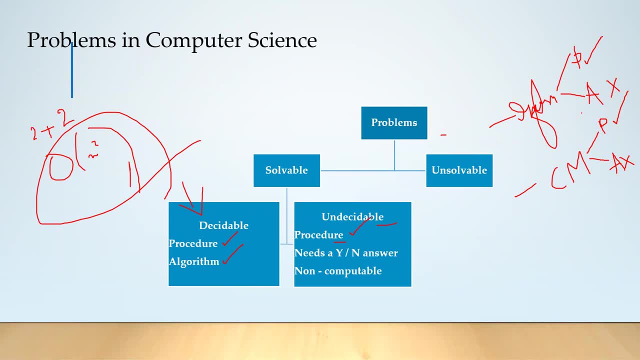 your first attempt. no, you can't say yes. your first attempt. no, you can't say yes or no, like you know or no, like you know or no, like you know, undecidable, you're not very sure. undecidable, you're not very sure. undecidable, you're not very sure, because you know you don't have a 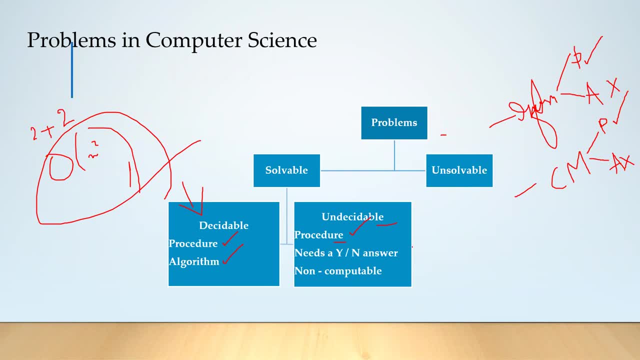 because you know you don't have a, because you know you don't have a, mathematics for that. mathematics for that. mathematics for that- undecidable. you need a yes or no answer. undecidable. you need a yes or no answer- undecidable. you need a yes or no answer, but unable to give it. 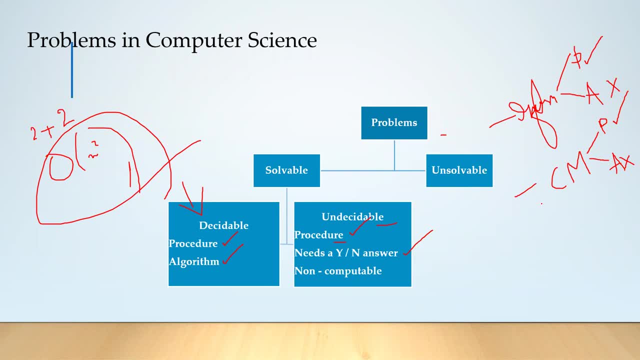 but unable to give it, but unable to give it. can you become the chief minister of? can you become the chief minister of? can you become the chief minister of kerala within the next 10 years? you know how to do it, but you know you. you know how to do it, but you know you. 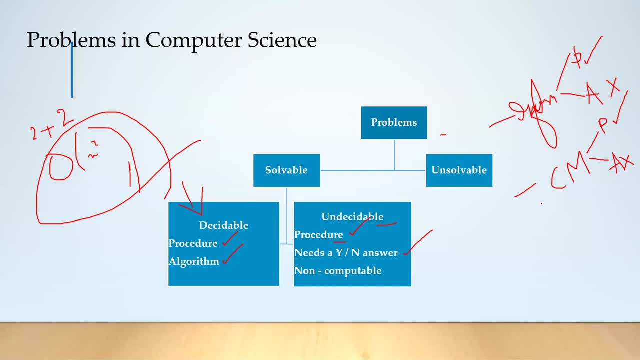 you know how to do it, but you know you don't know the time. don't know the time, don't know the time frame in which you will achieve it. you frame in which you will achieve it, you frame in which you will achieve it. you can't give me a yes or no answer, okay? 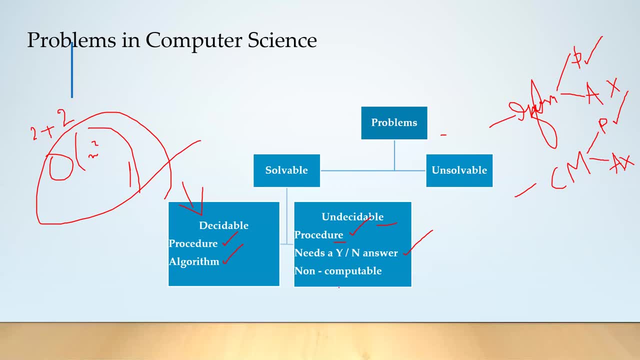 can't give me a yes or no answer, okay. can't give me a yes or no answer, okay. all those kind of problems, they come. all those kind of problems, they come. all those kind of problems, they come under undecidable problems, they are under undecidable problems, they are. 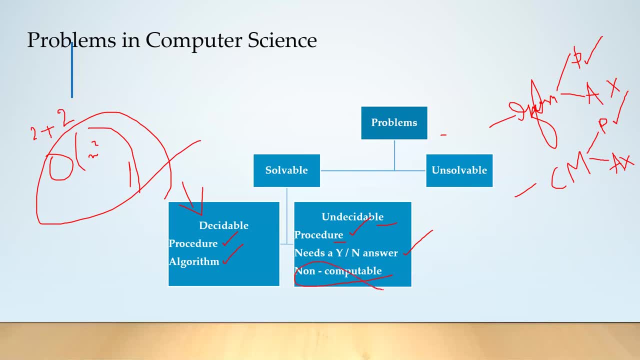 under undecidable problems. they are even called to be non-computable. you even called to be non-computable. you even called to be non-computable. you cannot compute it, or they're called cannot compute it, or they're called cannot compute it, or they're called non-computational problems. so very.